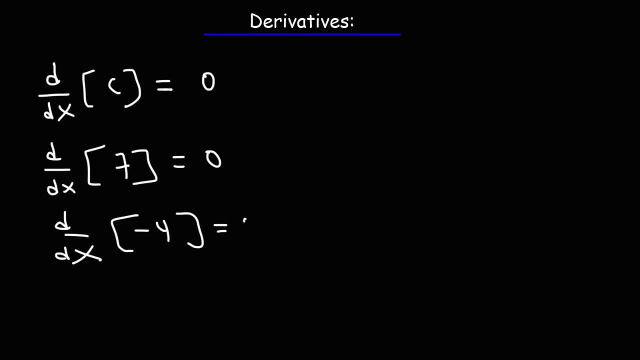 of a constant, like negative 4, that's also zero. Pi is just a number. there's no variable to it. so the derivative of pi is zero. The derivative of pi to the e, that's also zero. Both pi and e, they're just a number. So if you don't have a variable, if you just have a constant, the 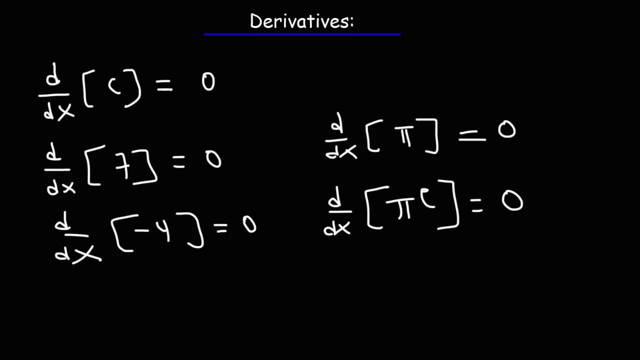 derivative of any constant is always zero. Now the next thing we need to talk about is something known as the power rule. Let's say: if we have a variable raised to a constant such as x raised to the nth power, This is equal to n times x raised to the n minus 1.. So let me give you some examples. Let's say we want to find the 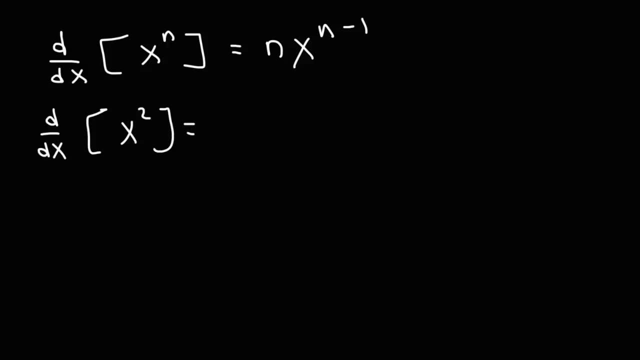 derivative of x to the second power, In this case n, is 2.. This is going to be 2 x raised to the 2 minus 1. Which is 2 x to the first power. In short, you need to move the exponent to the front and then subtract. 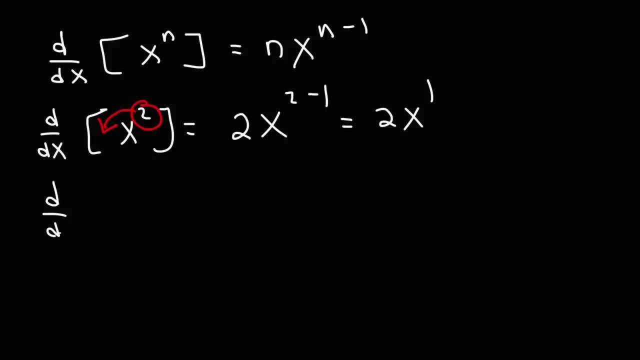 this by 1.. So let me give you some more examples. Let's say we want to find the derivative of x cubed, So what we're going to do is move the 3 to the front. So it's going to be 3, x, and then we're. 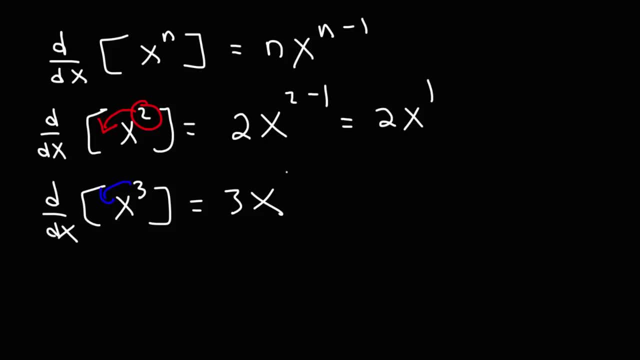 going to take away 1 from 3.. 3 minus 1 is 2, so it's 3 x squared. The derivative of x to the fourth, that's going to be 4 x cubed, And the derivative of x to the fifth power, that's 5 x to. 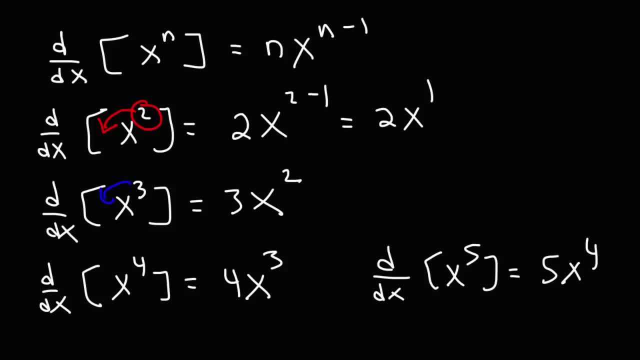 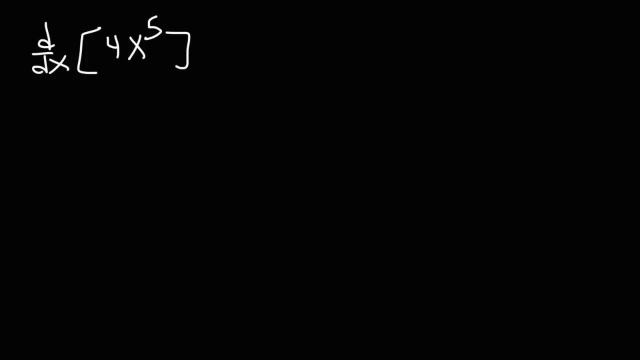 the fourth power. So hopefully you see the pattern here. but that's the power rule. That's how you can use it. So, with that in mind, what do you think the derivative of 4 x to the fifth power is equal to? So this is the same as the derivative of x to the fourth power. So let's say we want to find the 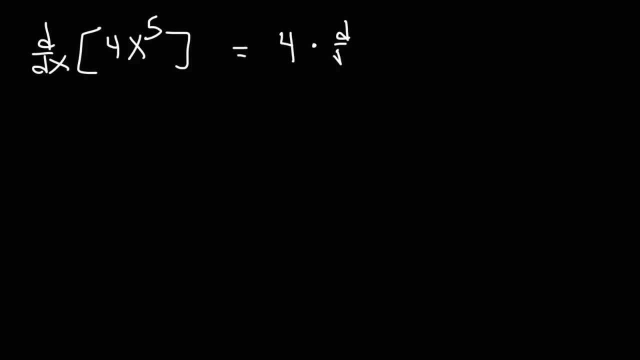 multiplying 4 by the derivative of x to the 5th power, And we could use the power rule on that part. The derivative of x to the 5th power is 5x to the 4th power, And then we could simply multiply 4 and 5. 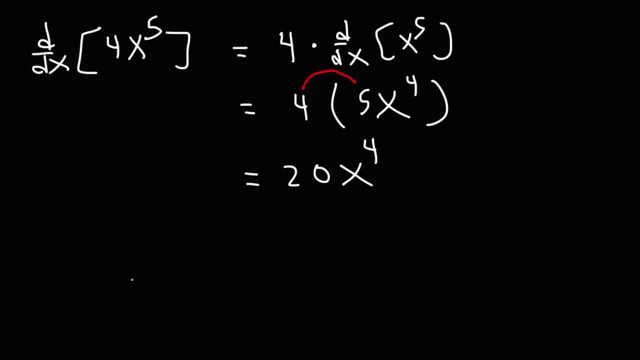 and this is going to be 20x to the 4th power. So this is known as the constant multiple rule. Go ahead and try these two examples: The derivative of 6x to the 8th power and also the derivative of 5x to the 3rd power. 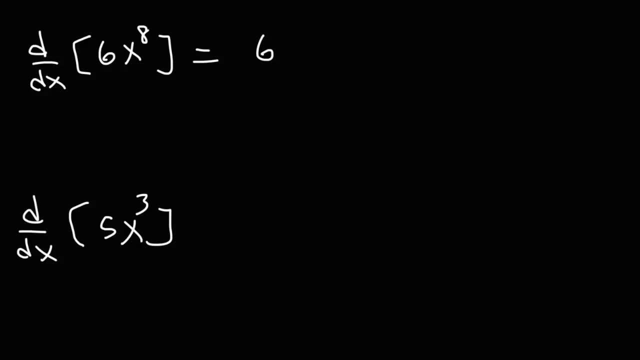 So let's start with the first one. We're going to rewrite the constant 6 and then multiply it by the derivative of x to the 8th power. So, moving the 8 to the front, it's going to be 6 times 8. 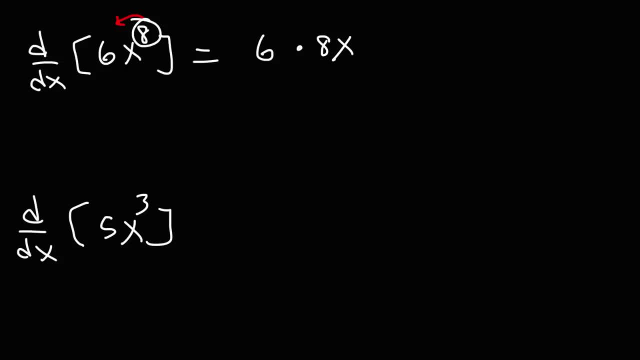 times x, and then we're going to subtract 8 by 1, which is 7.. So it's 6 times 8x to the 7th power, and then we can multiply 6 by 8.. That's going to be 48 times x to the 7th power. So that's the answer. 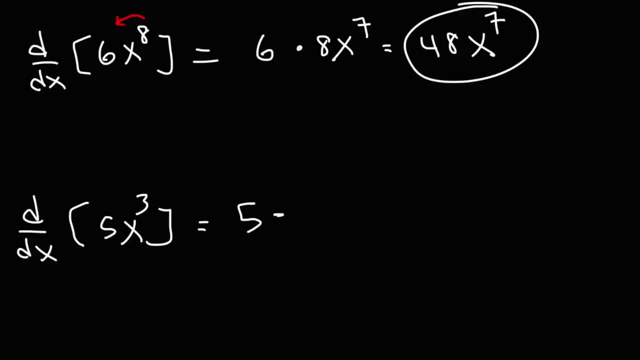 for the first example. For the second one it's going to be 5 times the derivative of x cubed, which is 3x squared, and then 5 times 3 is 15.. So the answer is 15x squared. Now let's say we have: 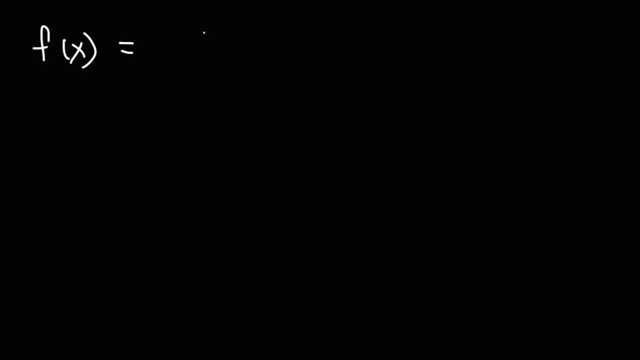 some polynomial function, f of x is equal to, let's say, 4x cubed plus 7x squared, minus 9x plus 5.. So what is the derivative of this function? By the way, the notation for the derivative of a function is: 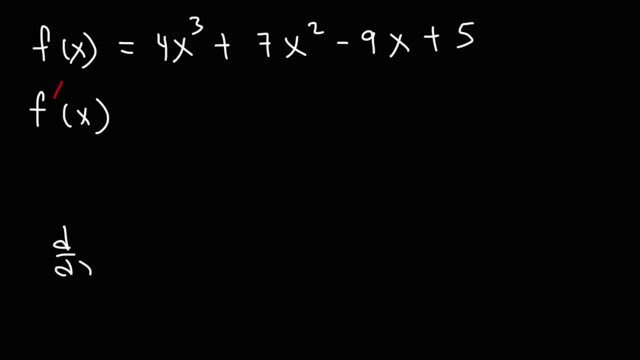 f prime of x. So if we take the derivative of f of x, this is going to equal f prime of x. for those of you who might be wondering. So for this problem we just got to take it one step at a time. 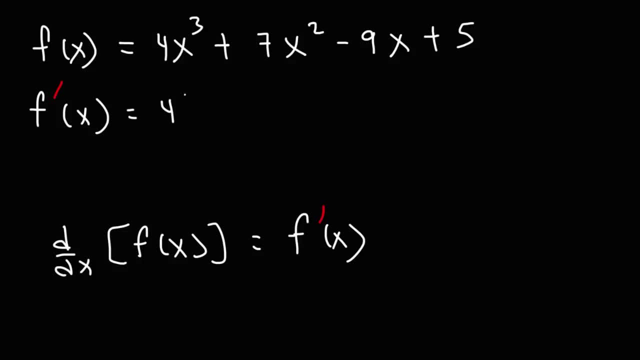 First let's find the derivative of 4x cubed. It's going to be 4 times the derivative of x cubed, which is 3x squared. And then next we need to find the derivative of 7x squared. 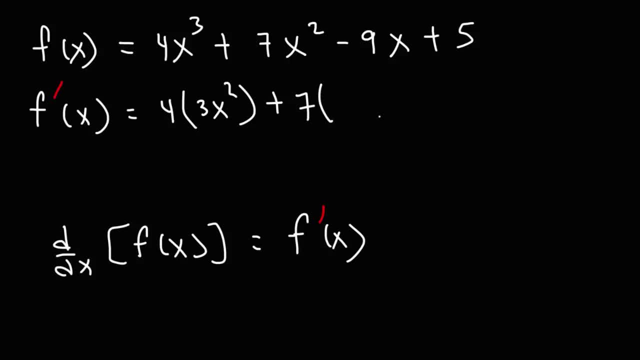 So it's going to be 7 times the derivative of x squared, which is 2x. Now what about the derivative of negative 9x? What is that equal to? Well, first we need to know what the derivative of x is equal to. 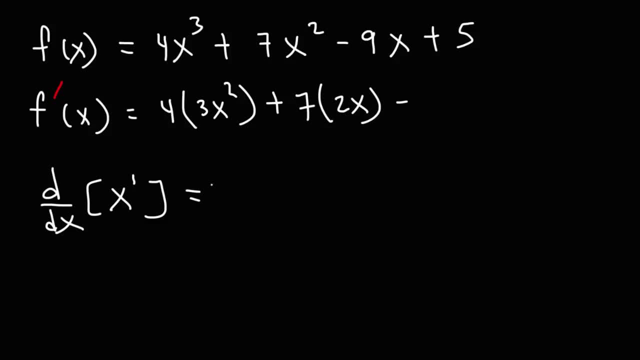 x is the same as x to the first power. So using the power rule, we can move the exponent to the front. It's going to be 1x And then if we subtract that number by 1, we get 0. 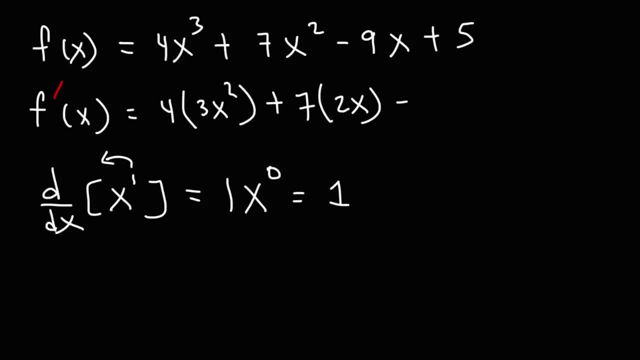 Anything raised to the 0 power is 1.. So the derivative of x, for instance, is 1.. The derivative of 5x is going to be 5 times 1, or 5.. The derivative of negative 7x is simply negative, 7.. So the derivative of negative 9x is simply. 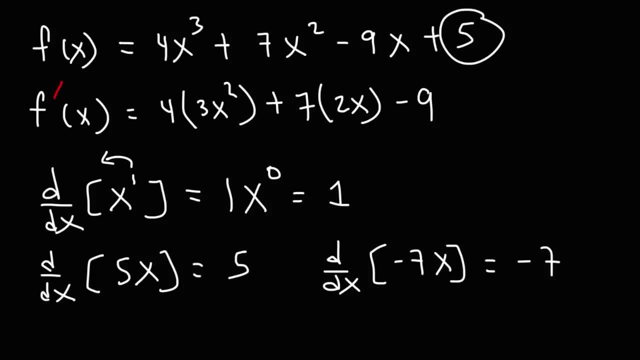 going to be negative 9.. And we know that the derivative of a constant, that is a number. without a variable, it's always 0. So the answer for this example is going to be 4 times 3, which is 12.. 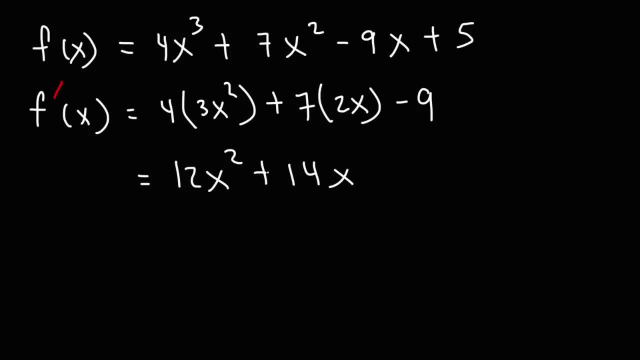 7 times 2 is 14.. And so it's going to be 12x squared plus 14x minus 9.. So that is the derivative of the original function. Now let's work on finding the derivative of a rational function. 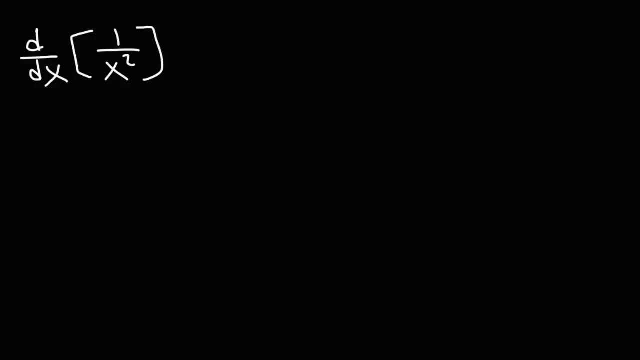 What is the derivative of 1 over x squared? How would you find the answer for this one? Well, it turns out that the derivative of 1 over x squared is 1 over x squared. It turns out that you could use the power rule, but you need to rewrite the expression first. 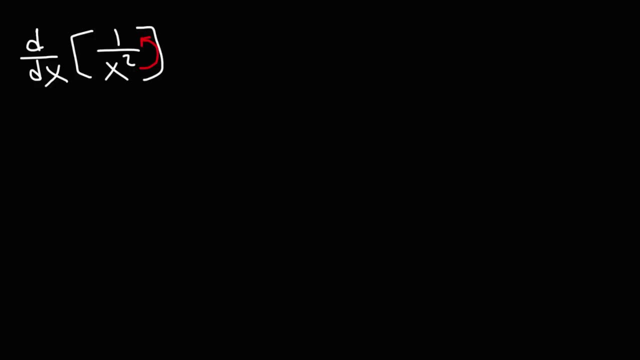 The first thing you need to do is move the x variable to the top. As you do so, the sine of the exponent changes from positive 2 to negative 2.. So you can write it like this, or you can simply just write it as x to the minus 2.. 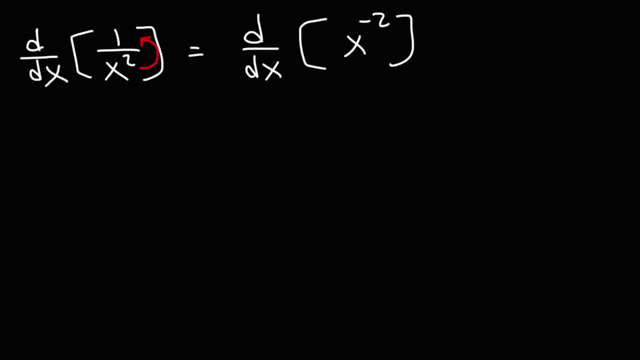 It's the same. So now, using the power rule, we can move the exponent to the front. This is going to be negative 2. x, and then we'll need to subtract the exponent by 1.. Negative 2 minus 1 is negative 3.. 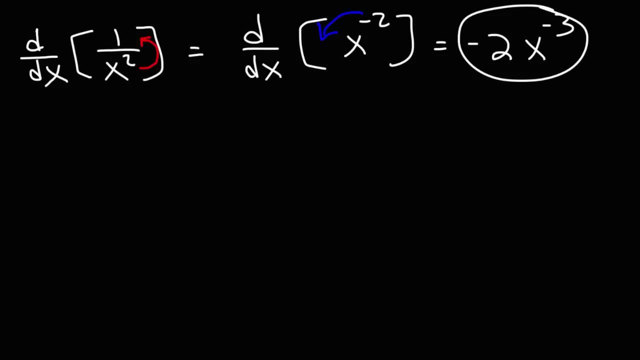 So this is our answer, but we can simplify it or rewrite it a bit. What you want to do is get rid of the negative exponent, So you want to move the x variable back to the bottom. Thus we're going to have a negative 2 on top and x raised to the positive 3 on the bottom. 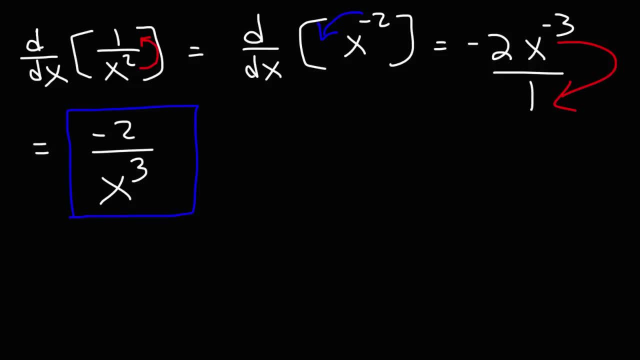 This is the final answer in its simplified form. So that's the derivative of 1 over x squared. Let's try another example. What is the derivative of 1 over x cubed? Feel free to pause the video if you want to work on it. 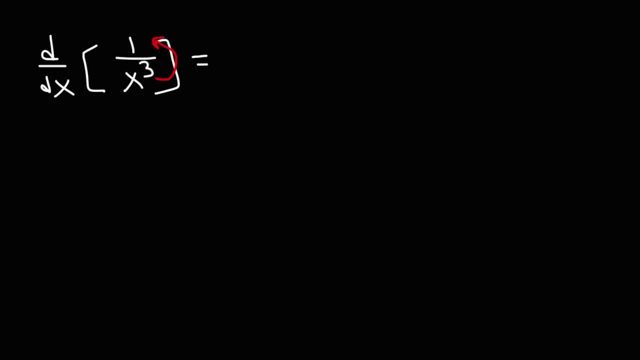 Step 1, we need to rewrite the expression. Let's move the x variable to the top, So this is equal to the derivative of x to the negative 3.. This is the derivative of x to the negative 3.. Now let's use the power rule. 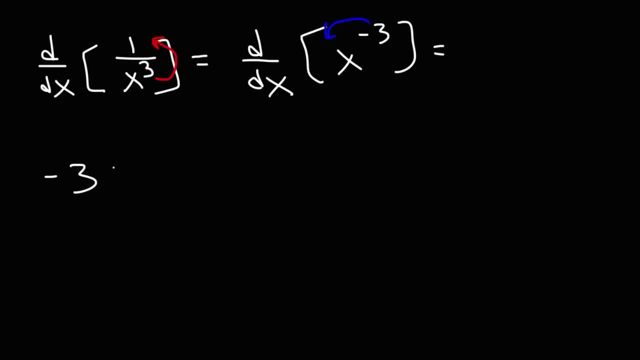 Let's move the exponent to the front, And so it's going to be negative 3x, and then let's subtract that number by 1.. So negative 3 minus 1 is negative 4.. Finally, let's move the x variable back to the bottom. 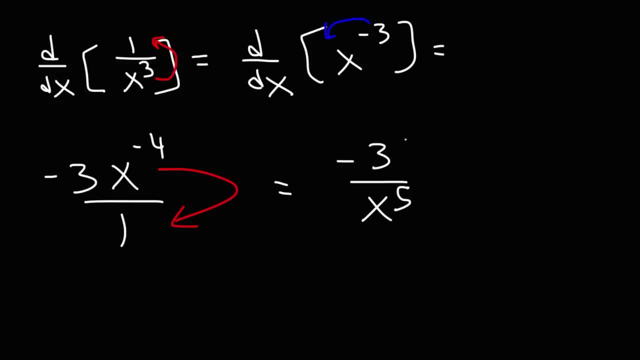 And so this is going to be negative 3 over x raised to the fifth power. Actually, I need to make a slight correction. That's negative 3 over x to the fourth power. That should be a 4.. So this, This is the answer to the problem. 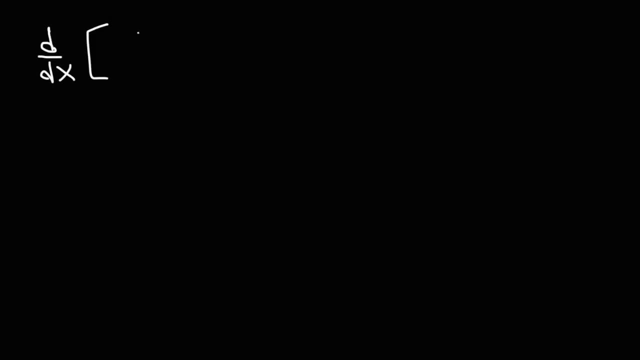 Now let's work on the next problem. Let's find the derivative of negative 6 over x to the fifth power. Go ahead and work on that. So, like before, we're going to move the x variable to the top. So the first step is to rewrite the problem. 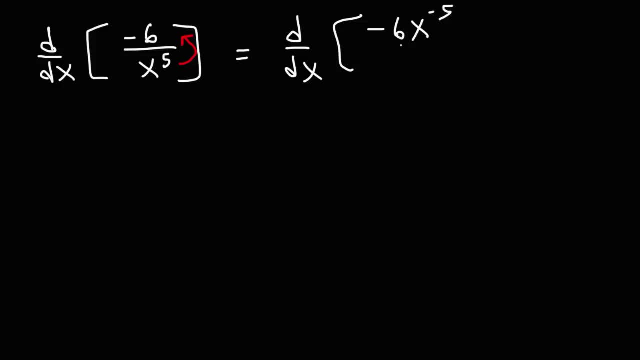 So this is going to be negative 6x to the negative fifth power over 1.. Now let's work on the next problem. So let's move the exponent to the front, So we're going to have negative 6 times negative 5, and then it's going to be x. 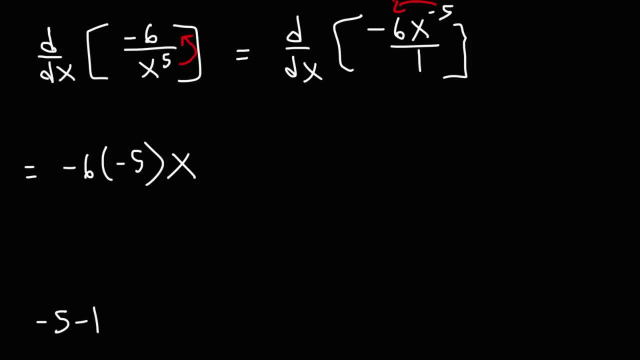 And then let's subtract negative 5 by 1.. Negative 5 minus 1 is negative 6.. So what we're going to do next is we're going to move the x variable back to the bottom and we're going to multiply those two numbers. 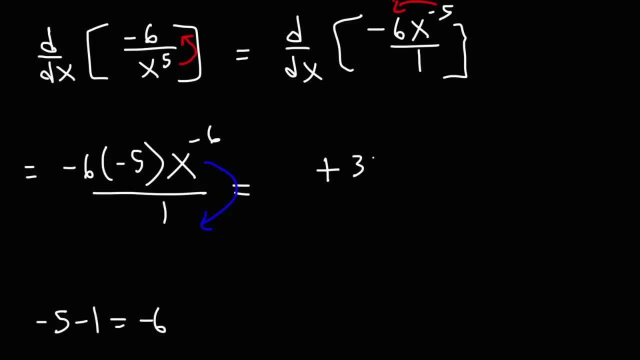 Negative 6 times negative 5, that's positive 30. And we have x to the 6 on the bottom. So this is the derivative of negative 6 over x to the fifth power. So now you know how to find the derivative of a rational function. 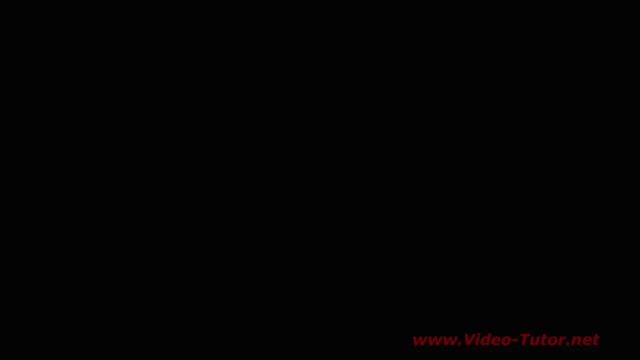 Let's move on to finding the derivative of a radical function. What is the derivative of the square root of x? How can we find the answer to that? Well, it's important to know that the x, the exponent, is 1, and the index number is 2.. 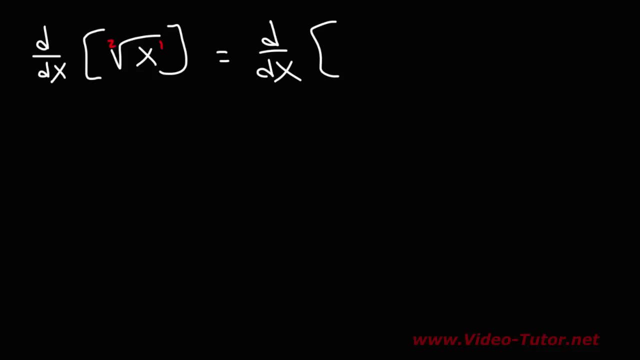 So, like before, we need to rewrite this problem. We can rewrite the square root of x as x to the 1 half. Now, in this form, we could use the power rule. So we're going to move the exponent to the front. 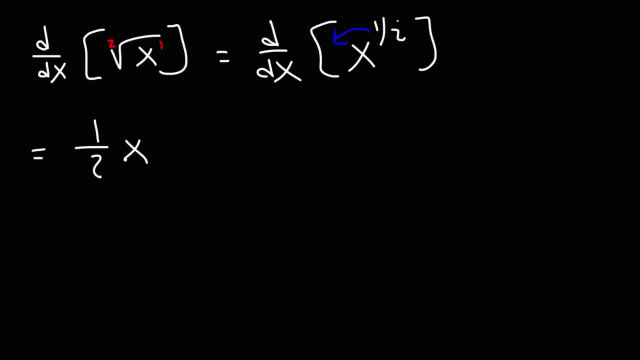 This is going to be 1 half x, And then we're going to subtract the exponent by 1.. So 1 half minus 1, we could change 1 to 2 over 2. So it becomes 1 minus 2, which is negative 1 over the same denominator of 2.. 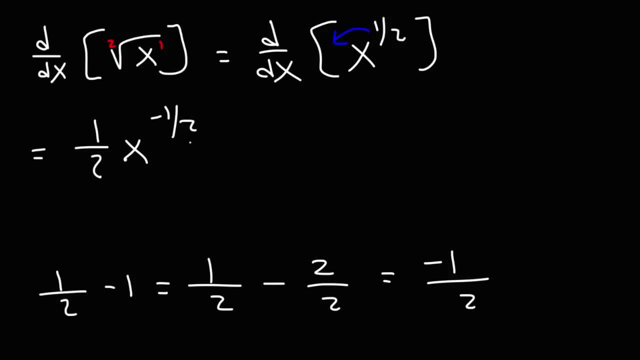 So 1 half minus 1 is negative 1 half. So now, at this point we can rewrite the expression. So this is equivalent to saying x raised to the negative 1 half divided by 2.. And now let's move the exponent- I mean the variable- back to the bottom. 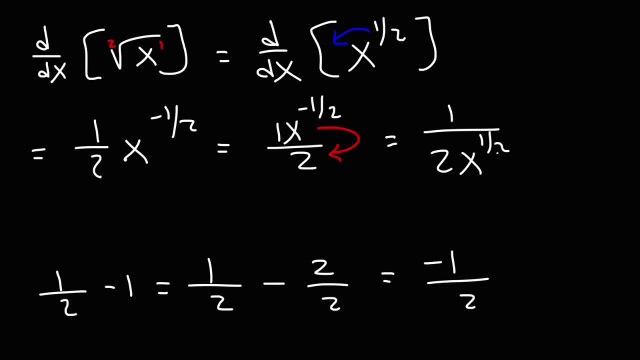 So it's going to be 1 half x. So it's going to be 1 over 2, x to the 1 half. And now, at this point, we can replace x to the 1 half with what we had at the beginning. 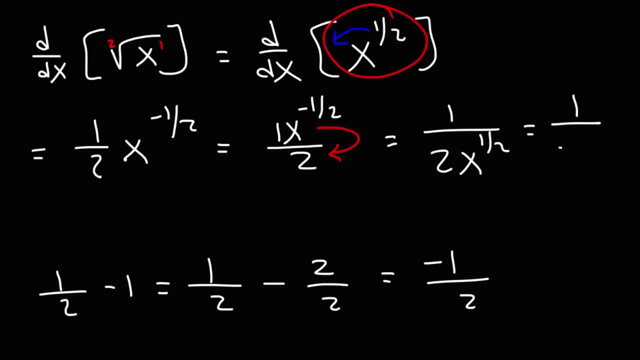 the square root of x. So the final answer is 1 over 2 times the square root of x. Now let's work on this example. Let's find the derivative of the cube root of x to the 5th power. Go ahead and take a minute to work on it. 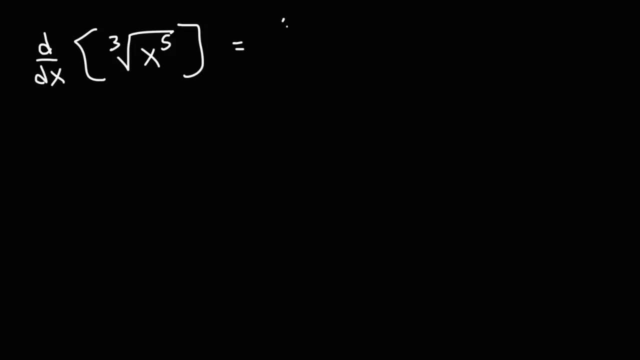 Feel free to pause the video, by the way, if you want to try any of these examples. So let's begin by rewriting the expression. The cube root of x to the 5th power is the same as x raised to the 5 over 3.. 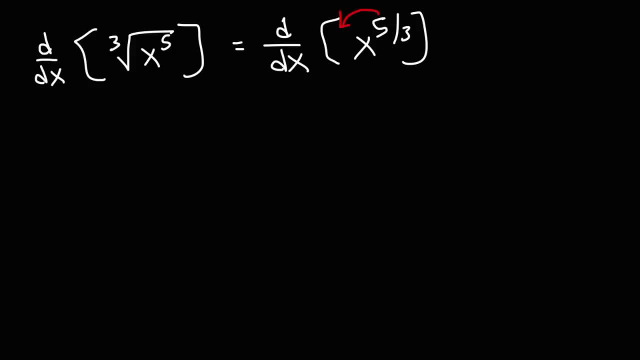 And now let's take the derivative by moving the exponent to the front. So it's going to be 5 over 3 x. and now we need to subtract that by 1.. So 5 over 3 minus 1.. Well, we need to get common denominators. 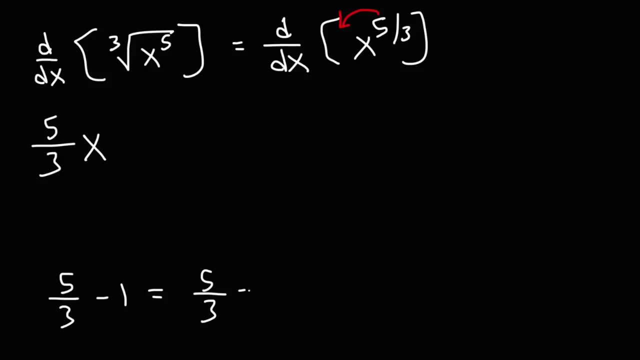 We're going to subtract these two numbers, So we're going to change 1 into 3 over 3, because 3 divided by 3 is 1.. And now we can subtract the numerators of the two fractions: 5 minus 3 is 2, and the denominator is going to stay the same. 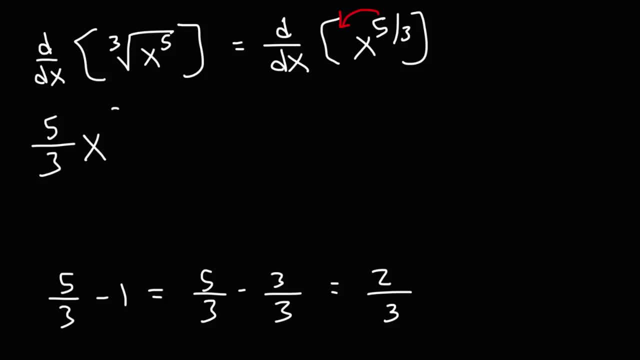 So 5 over 3 minus 3 over 3 is 2 over 3.. That's going to be our new exponent, And so you can move this x to the top and write it as 5 x raised to the 2 thirds divided by 3.. 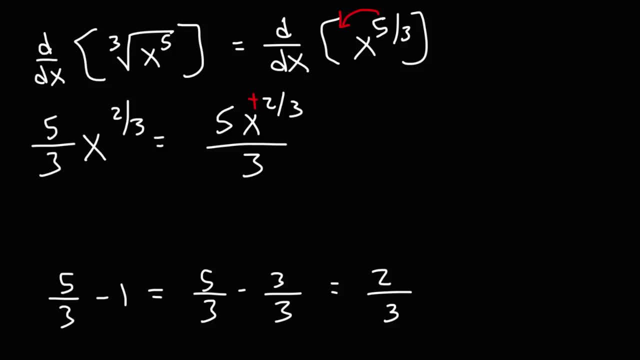 5 x raised to the 2 thirds, divided by 3.. Notice that we have a positive x point, So we're not going to move the x variable to the bottom and get a negative x point. There's no need to do that in this problem. 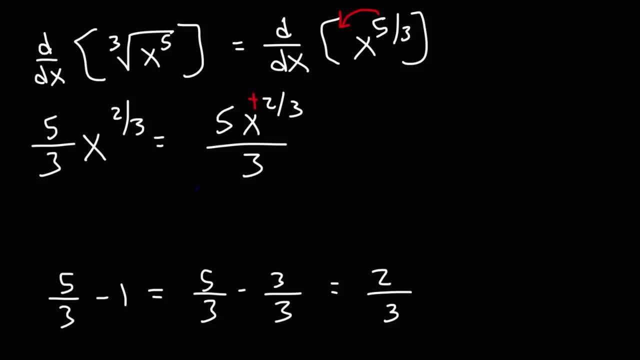 The only thing that we do need to do is convert this expression from an exponential fraction into a radical expression. So x raised to the 2 thirds can be rewritten as the cube root of x squared. So make sure you understand this. The b root of x to the a is equal to x raised to the a over b. 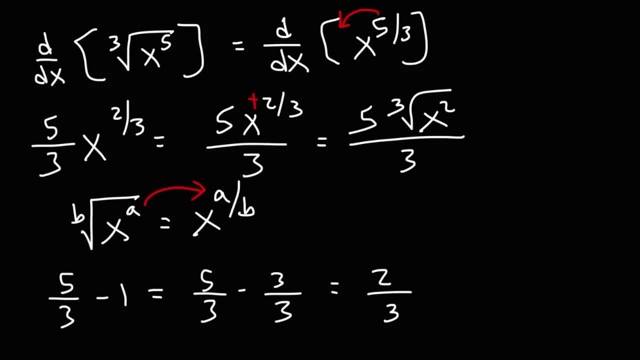 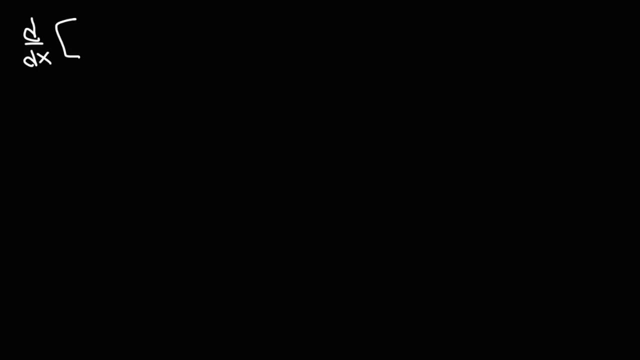 The number inside the radical goes on top of the fraction, The index number goes on the bottom of the exponential fraction. But for this problem this is the final answer. Now let's work on one more example of differentiating radical functions. So let's say we have the a-th root. 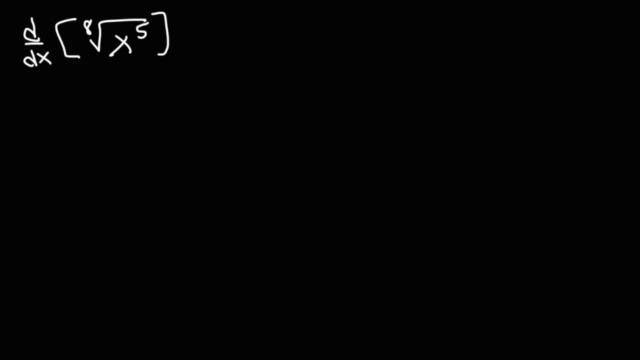 Of x to the 5th power. Go ahead and find the derivative of that. So let's begin by rewriting the expression. So the a-th root of x to the 5th is the same as x raised to the 5 over 8 power. 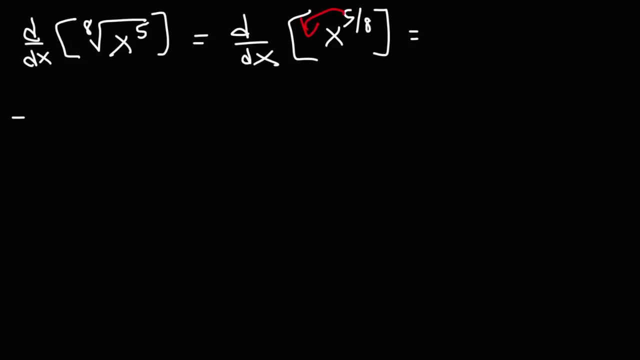 So now we're going to move the exponent to the front, just like before. This is going to be 5 over 8 x. Now let's subtract the exponent by 1.. We're following the same steps, So let's get common denominators. 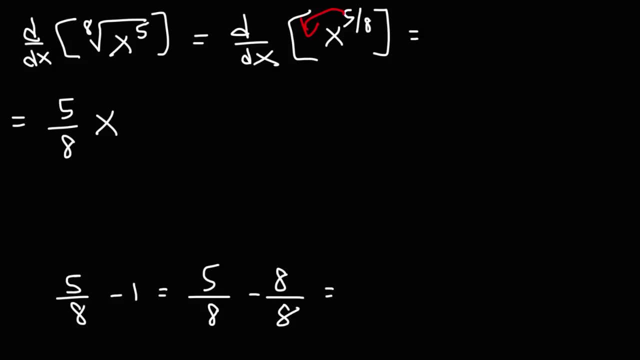 So let's replace negative 1 with negative 8 over 8.. 5 minus 8 is minus 3.. So this is going to be negative 3 over 8.. So we can rewrite this as 5x to the negative 3 over 8 over 8.. 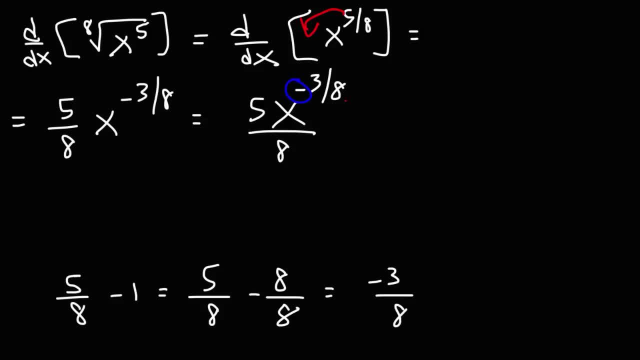 Now, this time we do have a negative exponent, So we're going to move the x variable to the bottom of the fraction. So it's 5 over 8, x raised to the 3 over 8.. Now the next thing we're going to do is convert the exponential fraction. 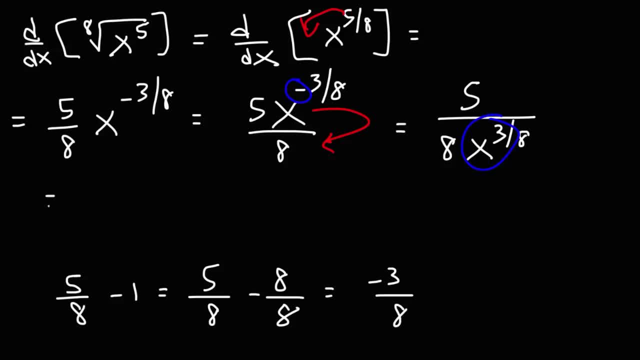 Back into its radical form. So x to the 3 eighths is the same as the a-th root of x cubed. Now we're going to leave the answer like this: Now, if you want to, you could rationalize the denominator. 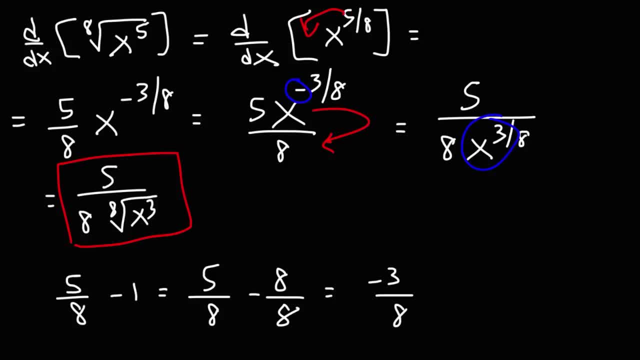 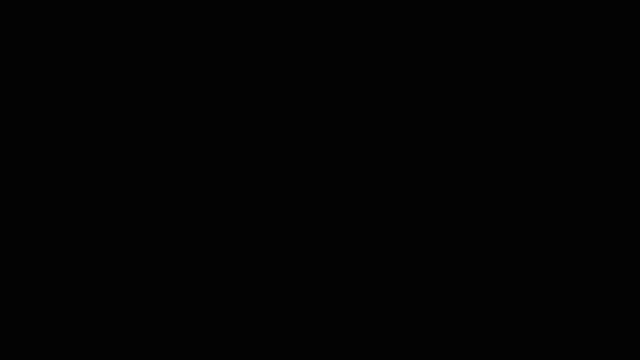 But that's a whole other topic. I'm going to leave the answer in this form. Now let's move on to finding the derivatives of trigonometric functions. So for now, hopefully you could take a look at this: Take out a sheet of paper and a pen or pencil and jot down some notes. 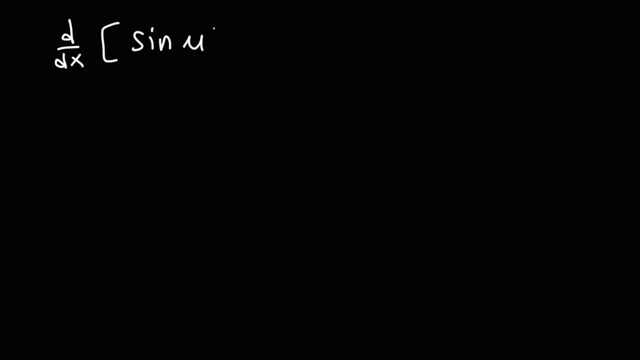 The derivative of sine of the u variable, where u is a function of x is going to be cosine of that u variable. times the derivative of u or times u prime. The derivative of cosine u is going to be negative sine of the u variable times u prime. 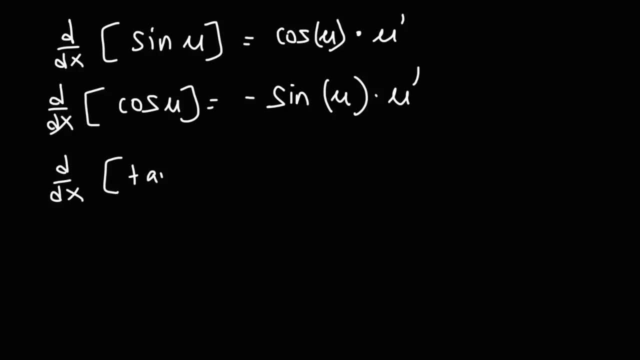 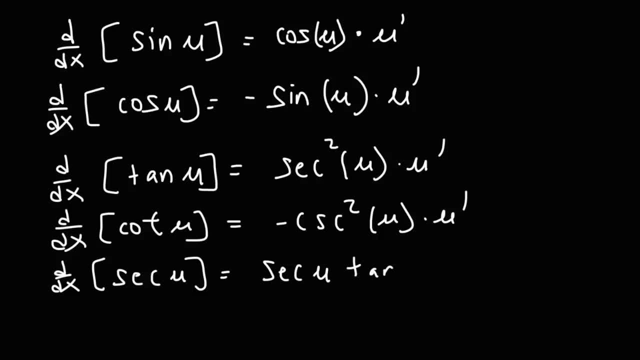 The derivative of secant is going to be negative: cosecant squared of u times u prime. So hopefully you see a pattern here. And finally, the derivative of cosecant is going to be negative: cosecant cotangent times u prime. So note that every time you differentiate a trig function that starts with a c. 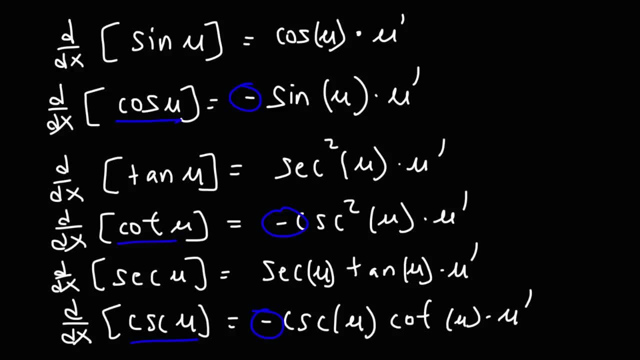 you're going to have a negative cosecant squared of u times u prime negative sign. That's one thing you want to keep in mind. The derivative of tangent and cotangent are similar to each other. This is secant squared, that's cosecant squared And the derivative of. 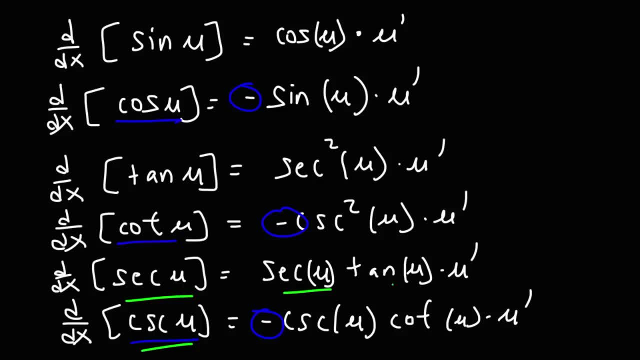 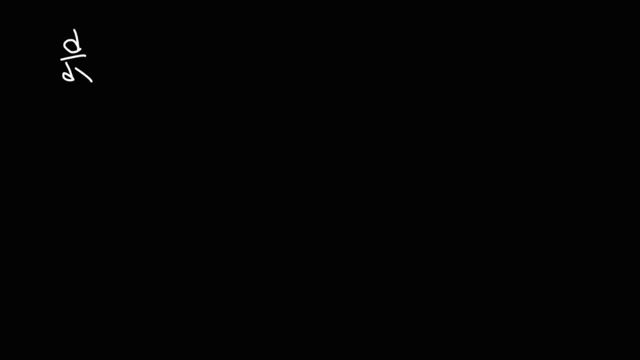 secant and cosecant are also similar to each other. This is secant tangent, this is cosecant cotangent. So hopefully that will help you to remember these trigonometric derivatives. Now let's try some example problems. Let's start with this one: What is the derivative of sine x? 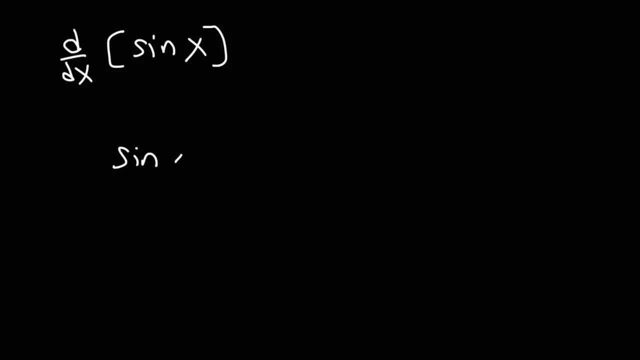 Well, we know that the derivative of sine to the u is going to be cosine u times u prime. In this example, we can clearly see that u is equal to x. If u is equal to x, what's u prime? Well, we know that the derivative of x is simply 1.. 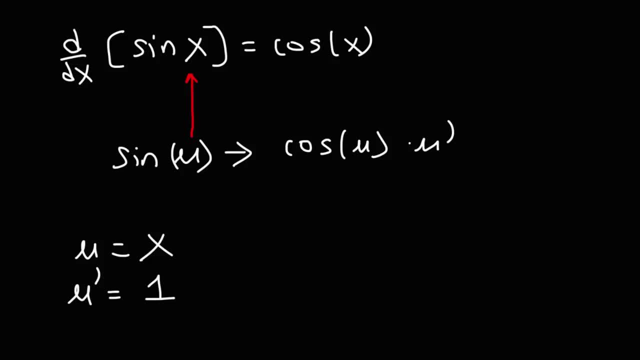 So this is going to be cosine x times 1, or just simply cosine x. Here's another example: What is the derivative of sine x to the third power? Try that one. So let's rewrite the formula: The derivative of sine to the u: it's going to be cosine of u times u prime. 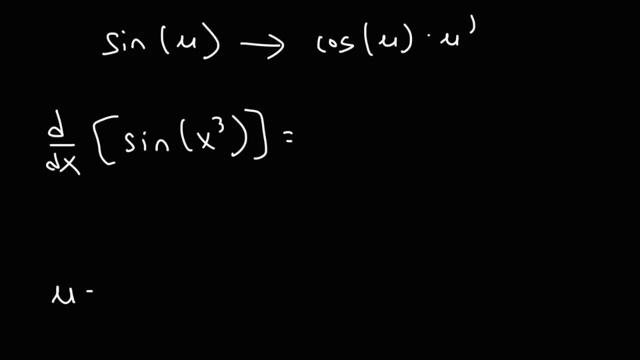 So the derivative of sine x cubed. well, first we know that u is x cubed, so u prime is going to be 3x squared, And then, if we just replace u with x cubed and u prime with 3x squared, we're going to 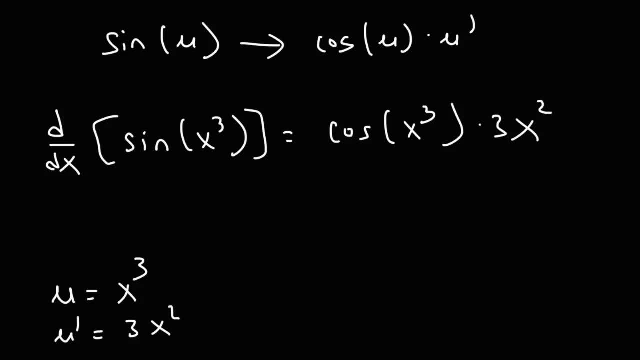 get the answer. So notice the process that we're taking here. First we differentiate sine. It turns into cosine, Whatever is inside of the sine function. that is the angle. It remains the same in the answer. So the angle of sine is x cubed. 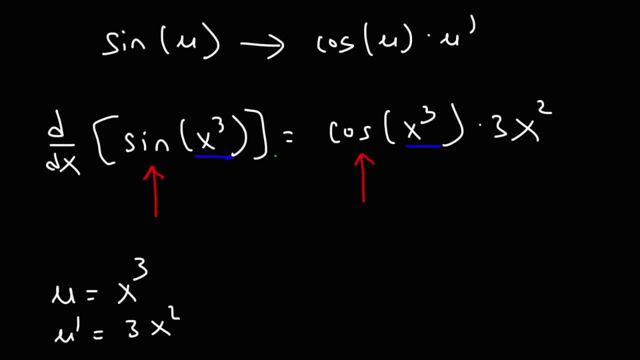 The angle of cosine remains x cubed. Next we take the derivative of the inside part of the function x cubed, and that gives us 3x squared. So now let's move on to some other examples. The derivative of cosine x squared. 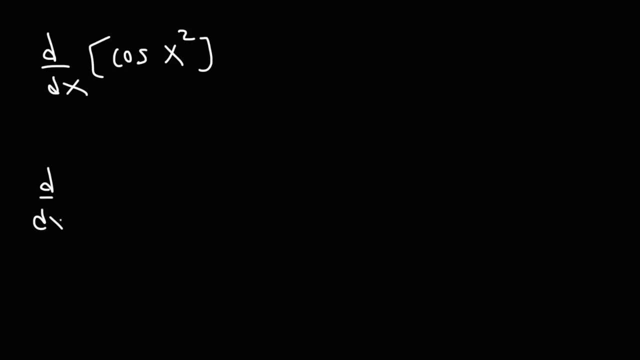 Try that one And also try the derivative of tangent Race to the x to the 5th power. I mean tangent of x to the 5th power. So first we're going to find the derivative of cosine. The derivative of cosine is negative sine. 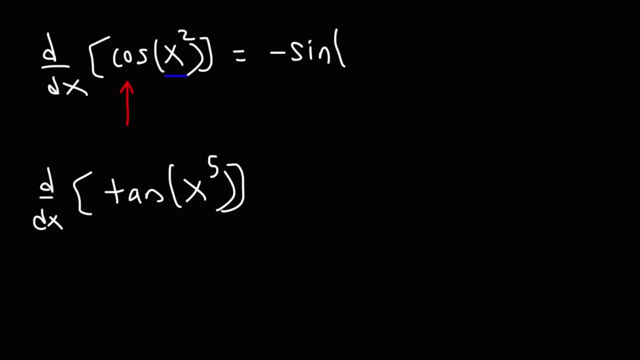 And we're going to keep the angle the same, So the angle is x squared. Next we're going to find the derivative of x squared, which is 2x. So the final answer is negative: 2x sine x squared. 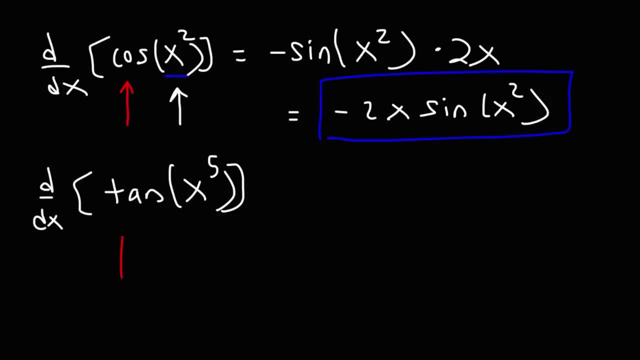 Now, moving on to the next example, the derivative of tangent is secant squared. Now, the angle of tangent is x to the 5th, So the angle of secant squared will be the same thing. Next, we're going to find the derivative of x to the 5th power, which is 5x to the 4th. 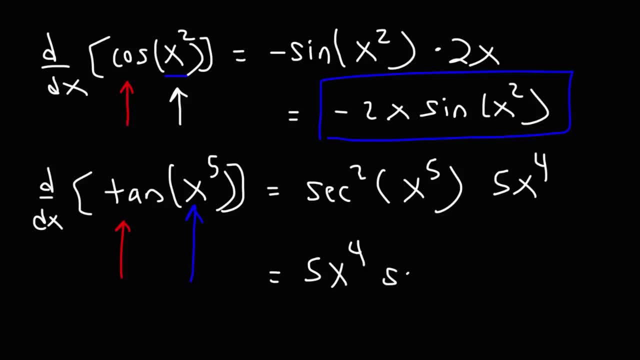 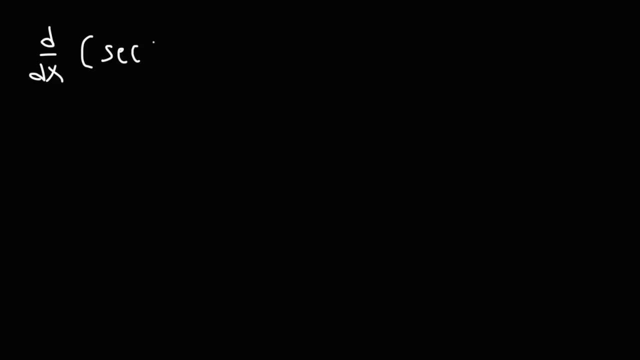 power. So the final answer is 5x to the 4th power times. secant squared x to the 5th power. Now what about the derivative of secant 4x? What's the answer to that one? The derivative of secant is secant tangent. 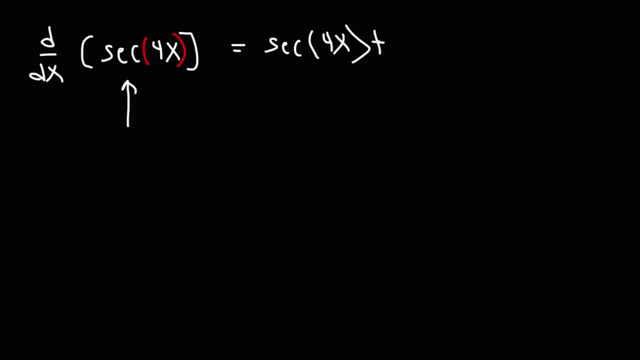 So it's going to be secant 4x, tangent 4x. The angle is going to remain the same. After that, we could find the derivative of 4x, which is just 4x to the 4th power. 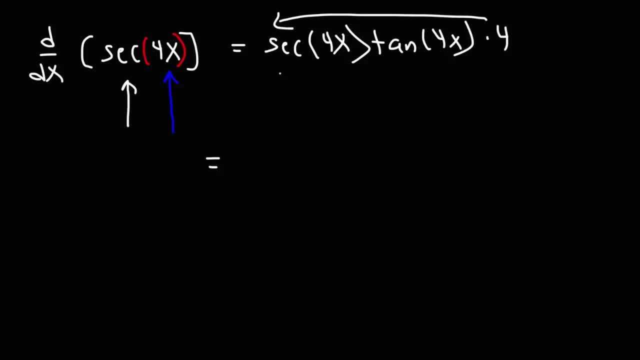 And I'm going to move the 4 to the front. So the derivative of secant 4x is going to be 4, secant 4x, tangent 4x. Now what about the derivative of, let's say, cotangent x cubed plus x raised to the 5th? 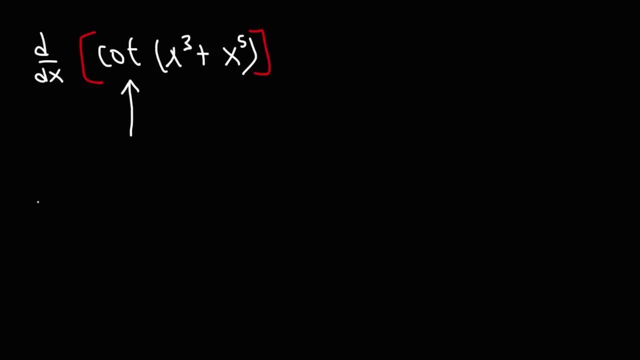 power. The derivative of cotangent is negative cosecant squared. So we're going to have negative cosecant squared And then whatever we have inside of the angle of cotangent, that's going to be the same for the angle of cosecant squared, which is x cubed plus x to the 5th power. 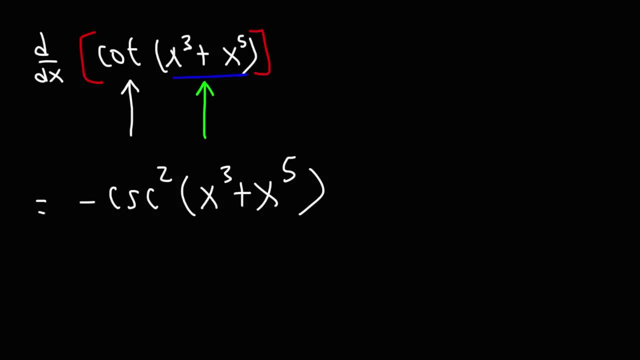 Next we need to find the derivative of the inside angle. The derivative of x cubed is 3x squared And the derivative of x to the 5th power is 3x squared, And the derivative of 5x to the 5th is 5x to the 4th. 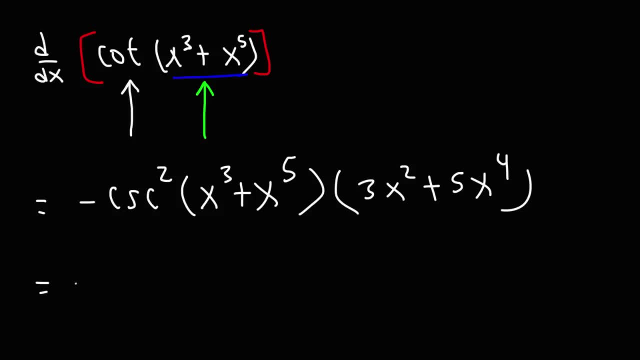 And so I'm going to leave the answer like that. But if you want to rewrite it, you could rewrite it like this: You could say: negative 3x squared plus 5x to the 4th power times: cosecant squared x cubed plus x to the 5th power. 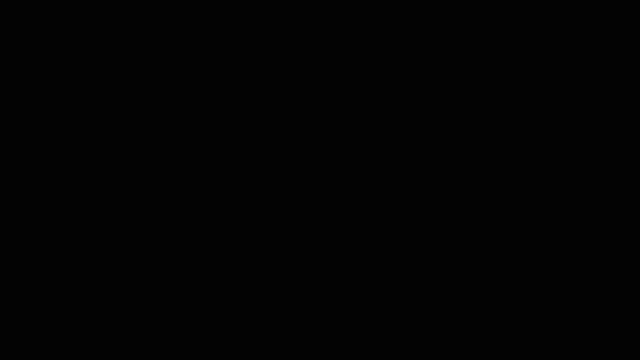 So that's the answer for this example. Now let's move on to the derivative Derivatives of natural logs. The derivative of ln, u: this is equal to u prime divided by u. So let's say, if we want to find the derivative of the natural log of x, 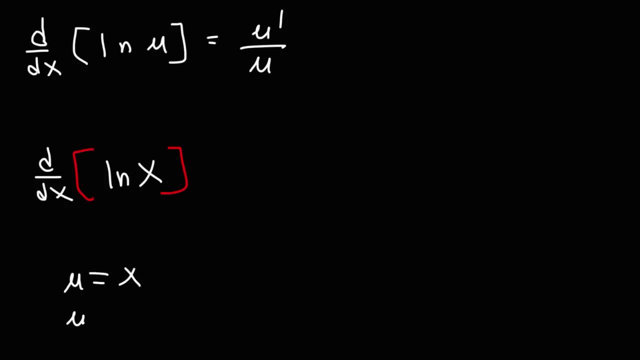 In this case, u is equal to x, u prime. the derivative of x is going to be 1.. So it's u prime over u or just 1 over x. So that's the derivative of the natural log of x. 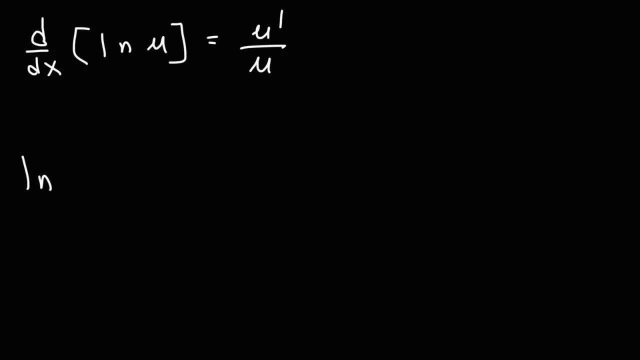 Now let's try some more examples. So what if we want to find the derivative of, let's say, the natural log of x cubed? What's the answer? Well, we can see that u is equal to x cubed. 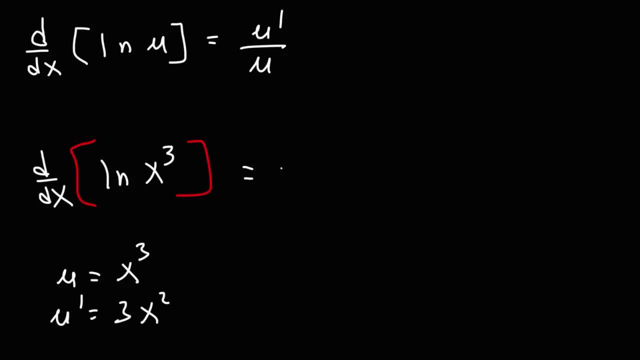 u prime is 3x squared, So it's u prime over u, That's 3x squared over x cubed. x squared is basically x times x. x cubed is x times x times x, So we can cross out two x variables. 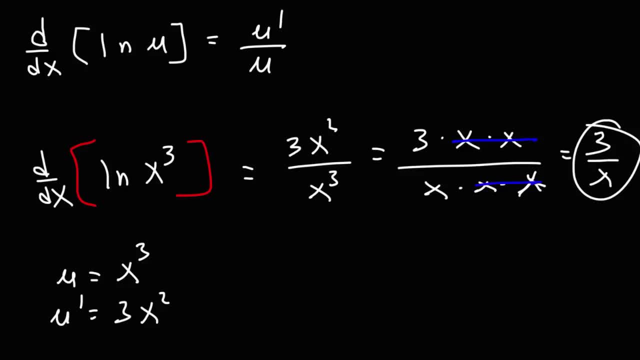 And this is going to give us 3 over x as a final answer. That's one way in which you can get the answer. Here's another way. A property of logs, and natural logs, allows you to move the exponent to the front. This is without differentiation, by the way. 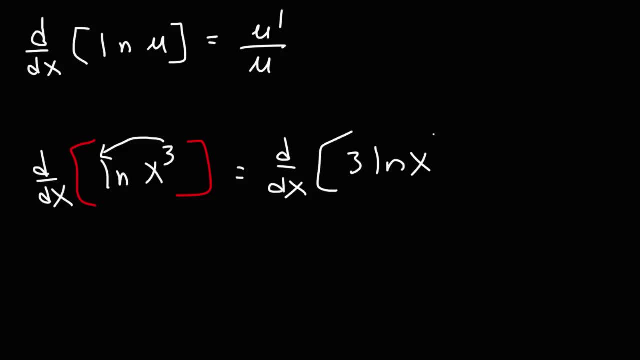 So we can rewrite the expression as Now. from the previous example we know that the derivative of ln x is 1 over x. So the derivative of 3 ln x is 3 times 1 over x, which is the same as 3 over x. 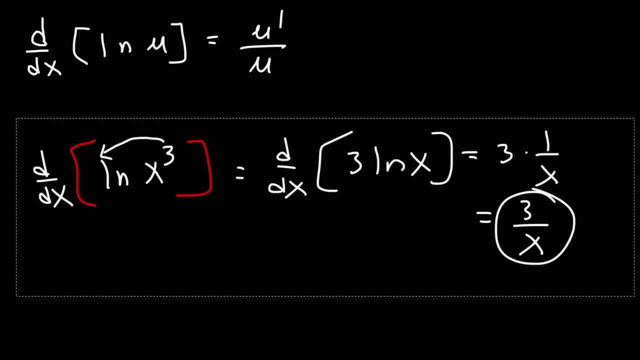 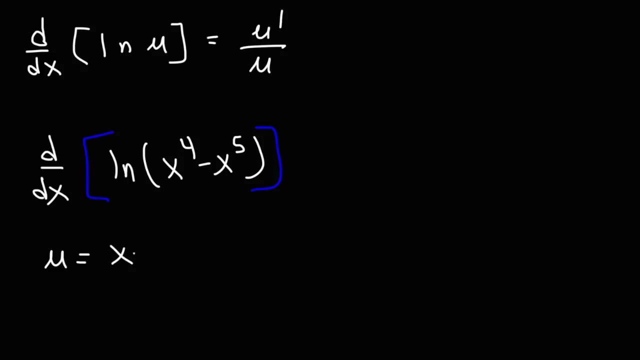 So that's another way in which you can find the derivative of that particular natural log function. Go ahead and try this one. Find the derivative Of ln, x to the 4th minus x to the 5th. So we can see that u is x to the 4th minus x to the 5th. 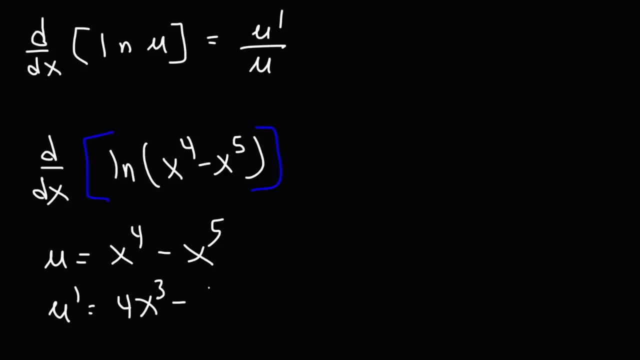 u prime is the derivative of that. It's 4x cubed minus 5x to the 4th. So the answer is going to be the derivative of what we see inside the natural log function divided by whatever is inside of it. 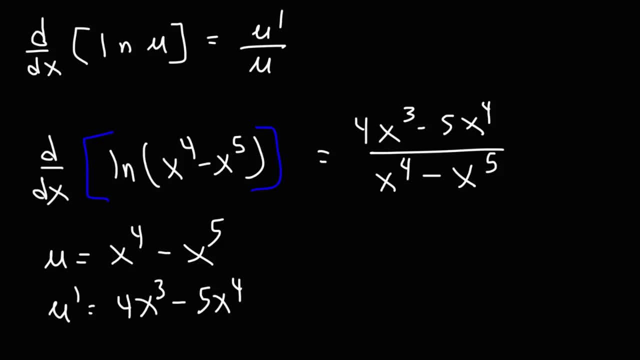 And that's really an easier way to like think about it in order to find the answer. So let's say, if we want to find the derivative of the natural log of tangent x, So first take the derivative of the inside part of ln. 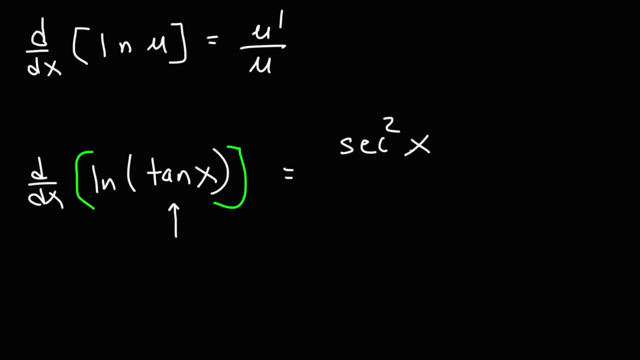 The derivative of tangent is secant squared And then simply divide it by whatever is inside of the natural log function which is tangent. So the answer is secant squared over tangent. But chances are we can reduce this expression. Secant is 1 over cosine. 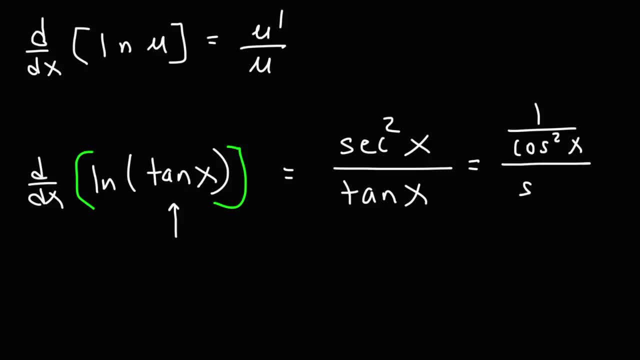 So secant squared is going to be 1 over cosine squared. Tangent is sine over cosine, So what we could do is multiply the top and the bottom by. I'm going to multiply it by cosine squared, These two will cancel and I'm going to get 1 on top. 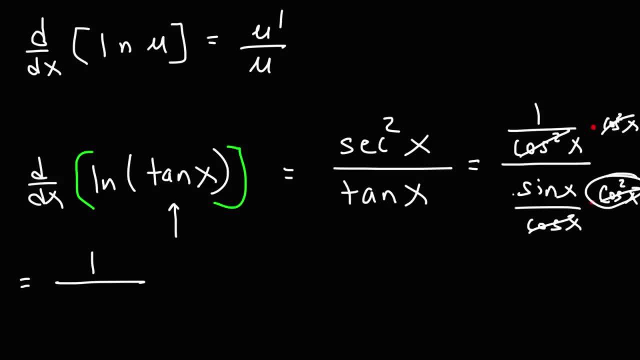 One of the cosines will cancel, leaving one cosine here. So I'm going to get sine times cosine, Which we can write that as: 1 over sine times, 1 over cosine, 1 over sine is cosecant x and 1 over cosine is secant x. 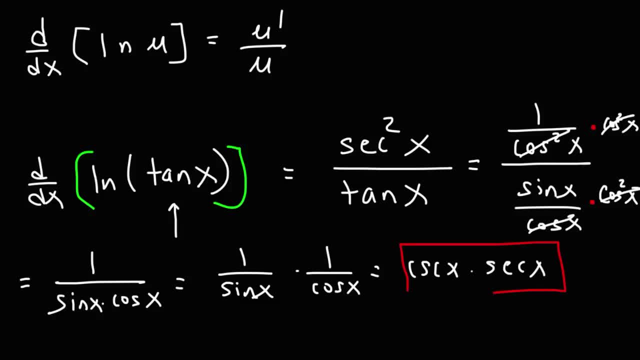 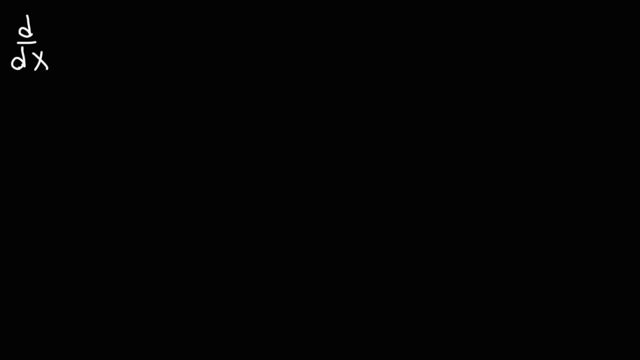 So the final answer is cosecant x times secant x. So now that we've talked about how to find the derivative of a natural log function, let's talk about how we could find the derivative of a regular logarithmic function, such as log base a of u. 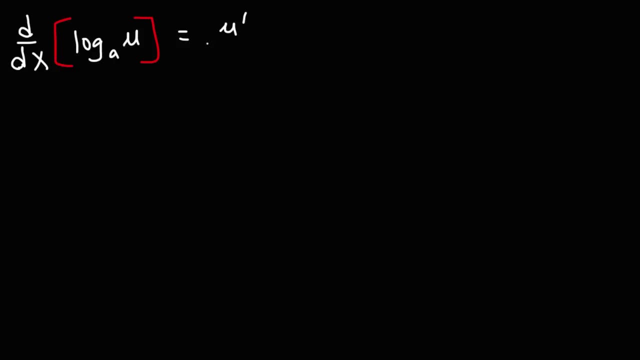 This is going to be equal to u prime over u, ln a. Now I'm going to compare that to the derivative of the natural log of u, Which we said is u prime over u. Now notice that here we have a base a and it turns into ln a. 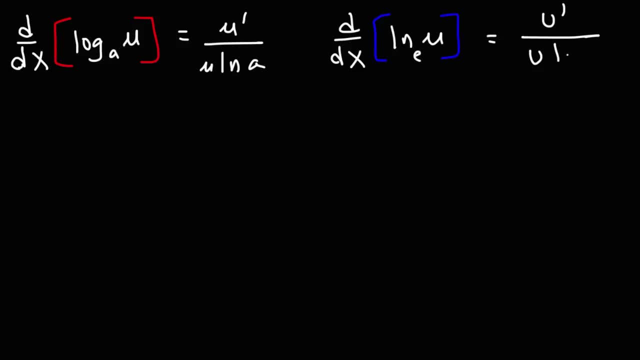 The base of a natural log is e, And what we should have here is l and e, So these two are essentially the same thing. Instead of a, we have e, But the natural log of e, what you need to know, is equal to 1.. 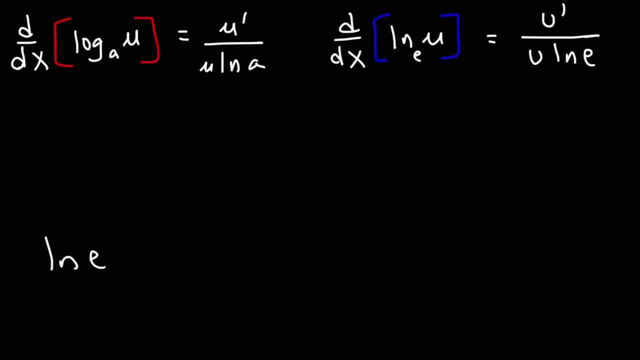 So because of that we really don't need this expression here. But I want you to compare and see the similarities between the two equations. So let's find The derivative of, let's say, log base 2 of x to the 5th power. 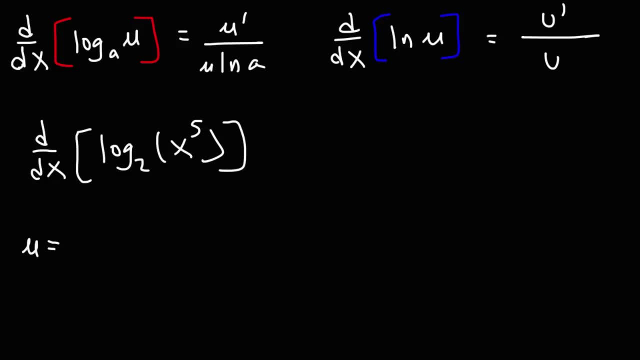 Go ahead and try that. u in this example is what we see here: x to the 5th power and a is 2.. u prime the derivative of x to the 5th power. that's going to be 5x to the 4th power. 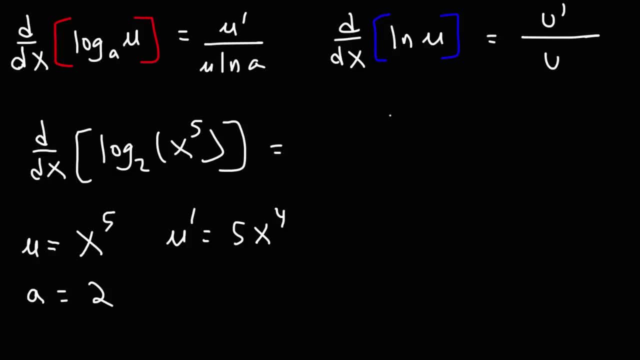 So all we've got to do Is plug in the information into that formula and we're going to get the answer. So it's u prime divided by u times the natural log of a or ln 2.. Now we can simplify our answer. 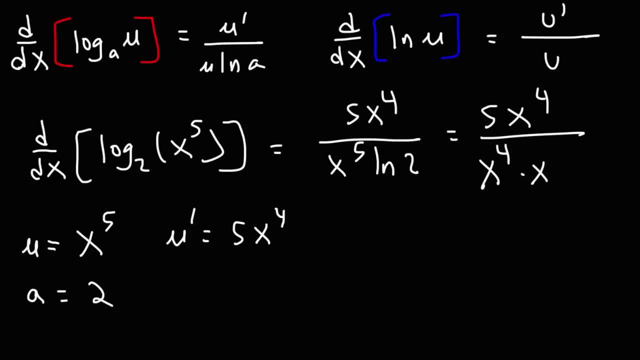 x to the 5th power. I can rewrite that as x to the 4th power times x, Because 1 plus 4 is 5. And so we can cancel x to the 4th power. Thus the final answer is going to be 5 over x ln 2.. 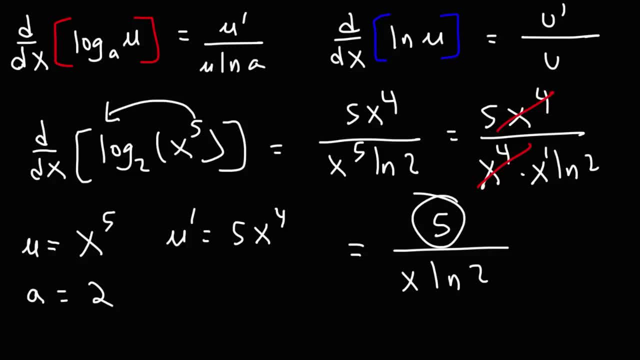 Now remember, you could move this 5 to the front, And thus we see that here. So that's the final simplified answer for that problem. Let's try another problem with regular logs. So let's say We have log base 4 of x cubed plus 4x squared. 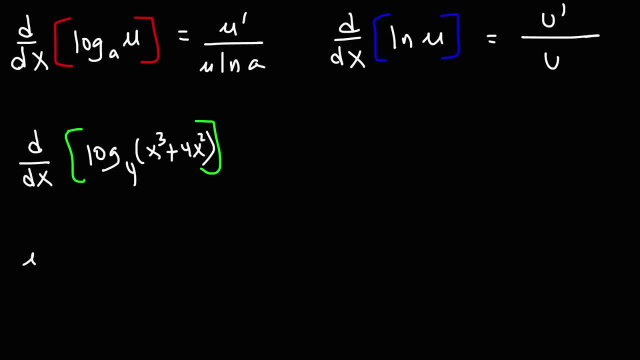 Let's try that one. So u is going to be whatever we see inside of the log expression. So it's x cubed plus 4x squared. a is the base of the log expression, a is 4. And u prime is just the derivative of what we see inside of here. 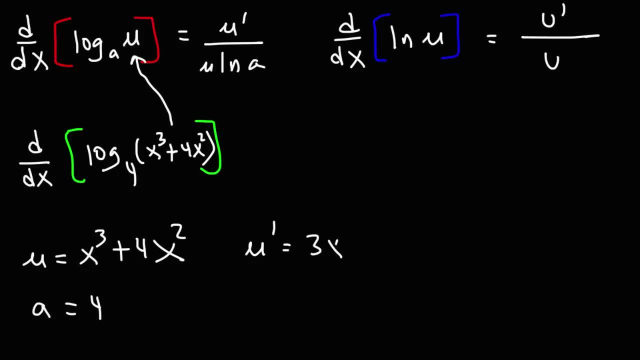 The derivative of x cubed is 3x squared. The derivative of 4x squared is 4 times 2x or 8x, And so, plugging everything into that formula, it's going to be u prime, which is 3x squared plus 8x. 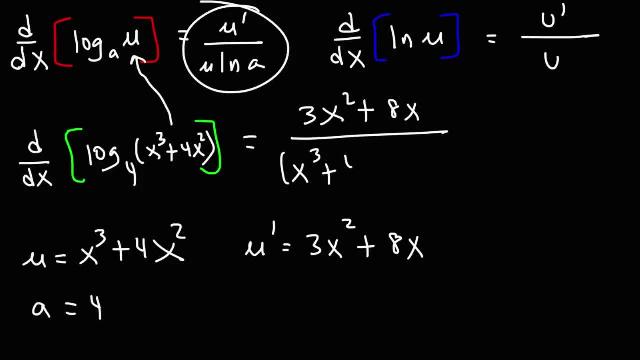 Divided by u, which is x cubed plus 4x squared, And then times the natural log of a or ln 4.. Now you can leave your answer like that, But understand that you could simplify this expression. In the numerator we can factor out an x. 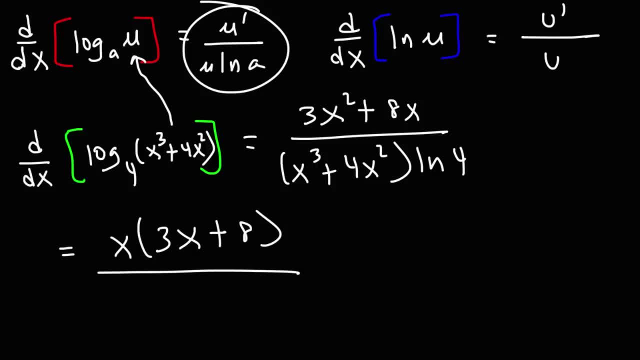 And we'll be left with 3x plus 8.. In the denominator we can take out an x squared, Which I'm going to write as x times x. If we take out x squared, we're going to be left with x plus 4.. 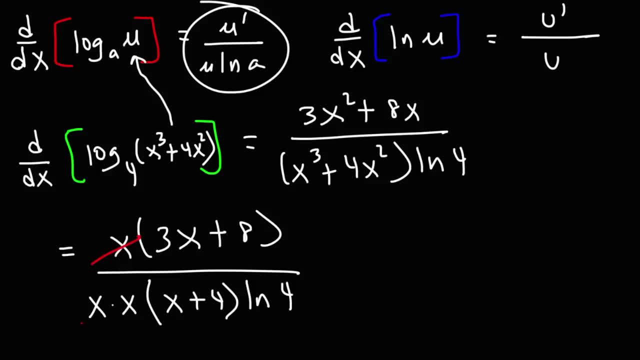 And then times ln, 4.. So now we can cross out an x variable, So we can leave our answer as 3x plus 8.. Divided by x times x plus 4, times the natural log of 4.. 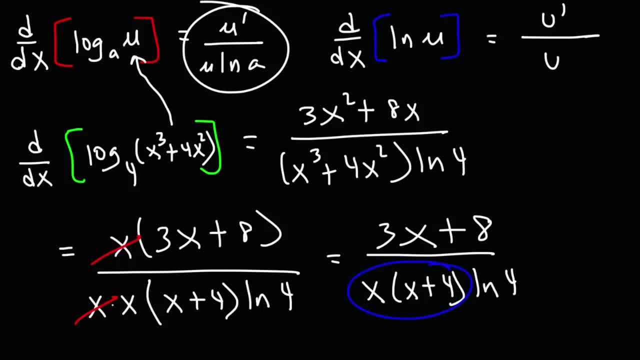 Or you can just rewrite that part as x squared plus 4x. There's many ways in which you can write your final answer. Hopefully, your teacher won't be too picky about exactly how she wants you to leave your final answer. 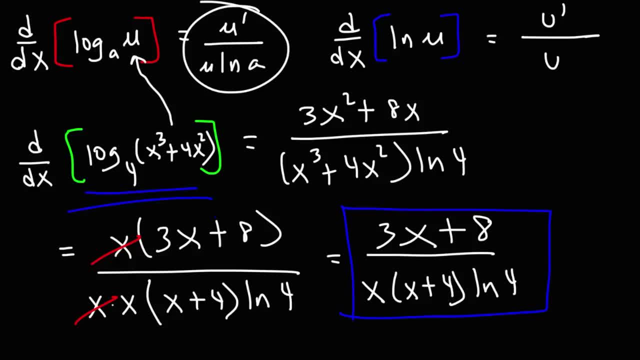 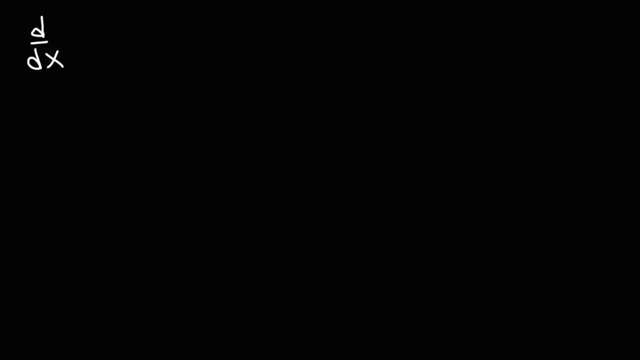 But that's it. So that's how you can find the derivative of this logarithmic function. Now let's move on. Let's move on to our next topic, And that is the derivative of exponential functions. So let's say we have a constant raised to a variable. 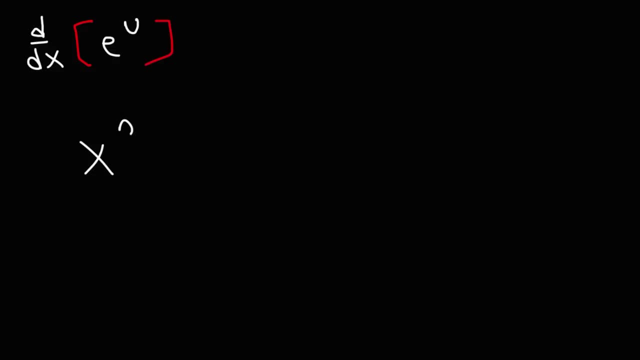 Before we had a variable raised to a constant which we would use the power rule, But now we have a constant raised to a variable And this is going to equal that constant raised to that variable times the derivative of that variable. 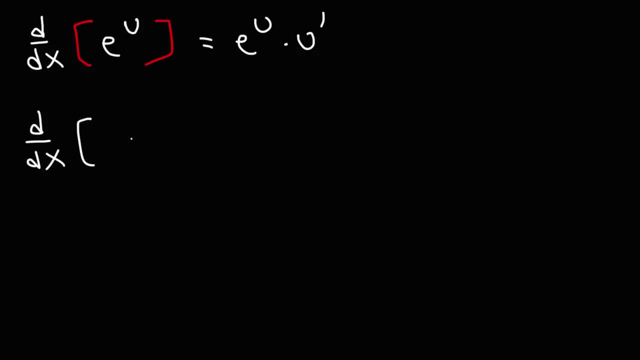 So let's put this information to practice. Let's say, if we want to find the derivative of e to the x, So it's going to be e to the x times the derivative of x, which is 1.. So the derivative of e to the x is simply e raised to the x power. 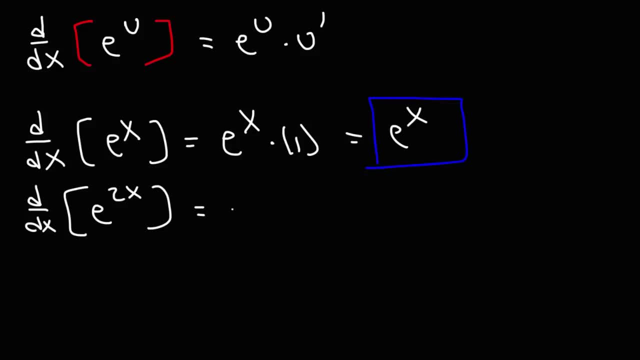 Now what about the derivative of e to the 2x? It's going to be the same thing: e to the 2x times the derivative of 2x, which is 2.. So you can write it as 2e to the 2x. 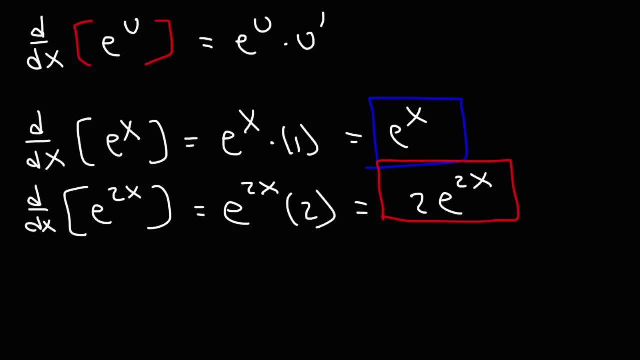 Now let's work on some other examples. What is the derivative of e to the 5x? It's going to be e to the 5x times 5, which is 5e to the 5x. And then, finally, if we have the derivative of e to the x squared, it's going to be the same thing: e to the x squared times the derivative of x squared, which is 2x. 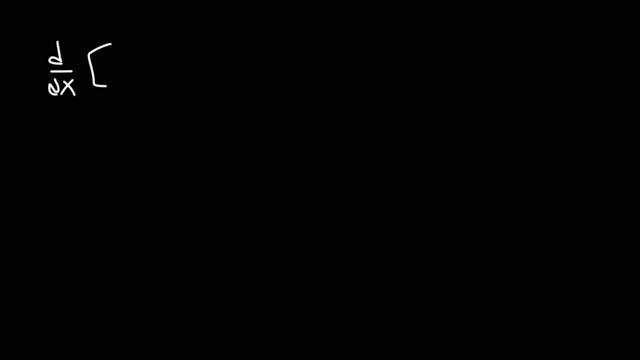 Now let's do one more. Let's say we want to find the derivative of e to the sine x. This is going to be e raised to the sine x times the derivative of sine x, which is cosine x. So that's how you can differentiate an exponential function with a base e. 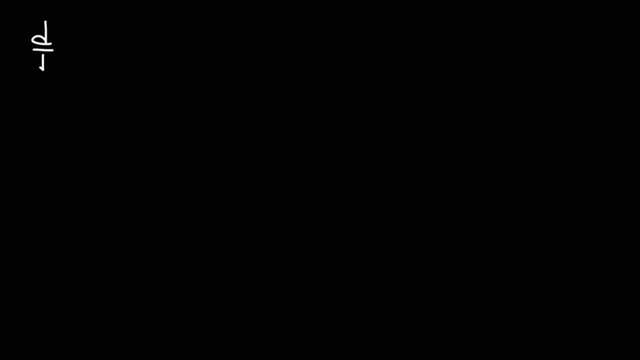 Now what if the base is not e? Let's say it's some number other than e, because e is a special number. It's equal to 2e, It's equal to 2.7182818, and it just continues. 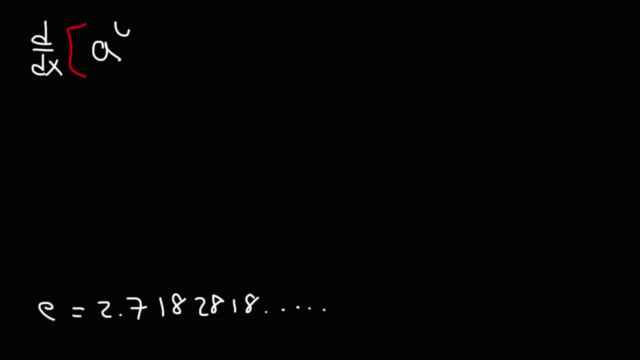 But what if we have, let's say, some other constant raised to the u variable? What's the derivative of that? It's going to be the same thing: a to the? u times u prime, but times ln a. If we contrast that with e to the u, which is e to the? u times u prime, but technically times ln e. 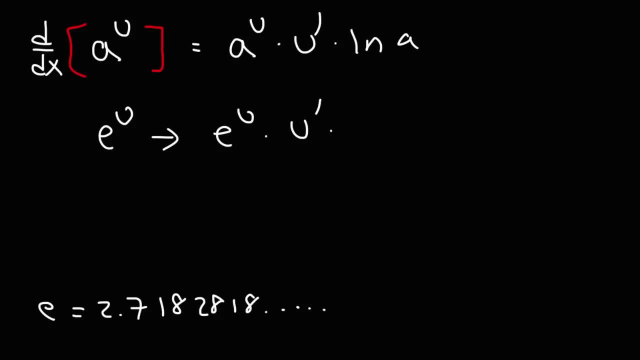 But ln e is 1? So we don't need that part when dealing with e. It's just e to the u times u prime. But if the constant is a number other than e, then you need to add the ln a part to the answer. 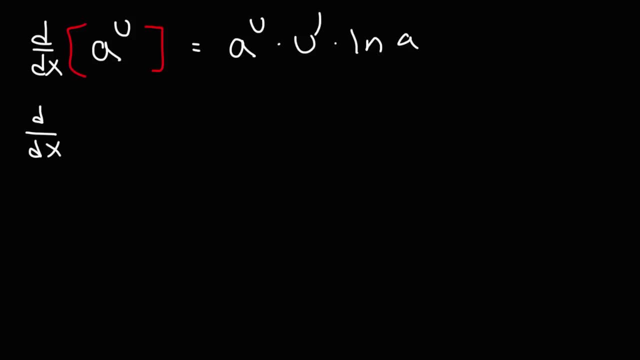 So let's put this to practice. Let's say we want to find the derivative of 5 raised to the x power. This is going to be the same thing: 5 raised to the x Times the derivative of x, which is 1, times the ln of 5.. 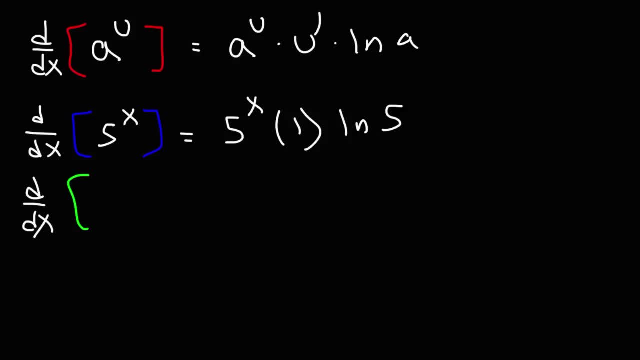 So, based on that, go ahead and try these examples: Find the derivative of 4 raised to the x squared, And also the derivative of 7 raised to the x to the 4th. So this is going to be whatever we see here. 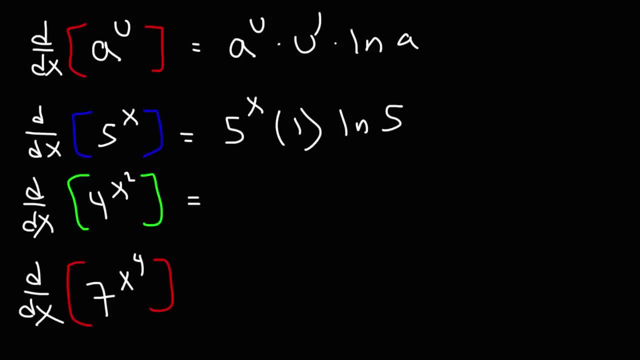 So we're just going to rewrite it. That's 4 raised to the x squared and then times u prime. u in this example is x squared, So the derivative of x squared is 2x, And then times the ln of whatever the base is. 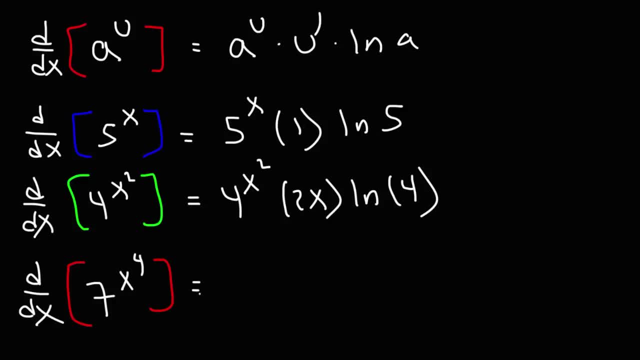 The base in this example is 4.. For the next one, it's going to be exactly what we started with: 7 raised to the x to the 4th Times. the derivative of the exponent, The derivative of x to the 4th, is 4x cubed. 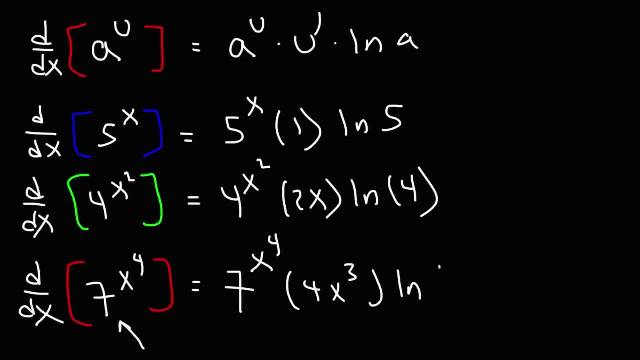 Times the natural log of the base, And the base is 7.. So that's the derivative of 7x to the 4th. You simply need to just follow the equation. As you can see. this is the a to the? u part. 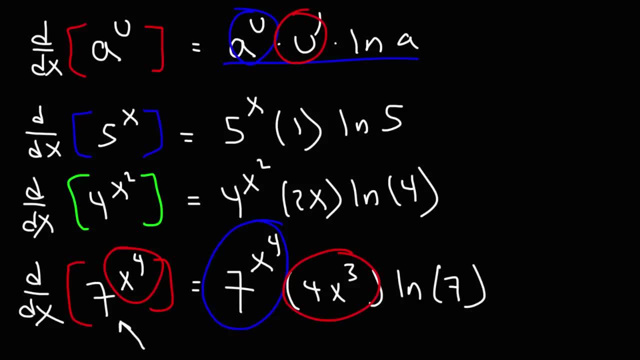 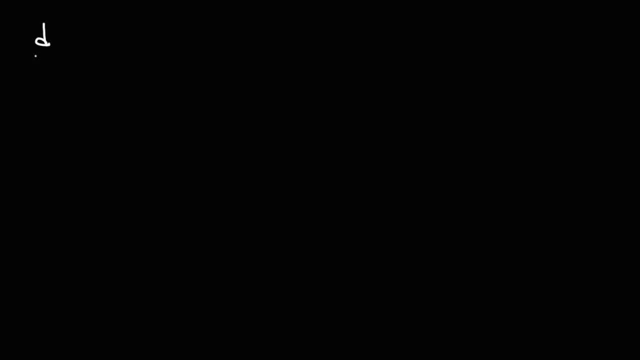 u, prime, that's the derivative of the exponent, And then ln, a. We can see a is 7.. Now the next topic of discussion is the product rule. So let's say you have a function multiplied to another function. 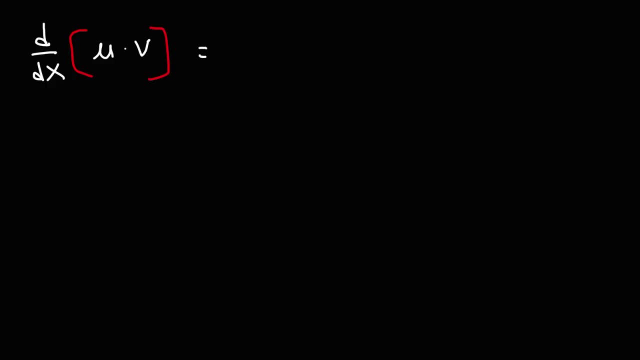 u times v. What is the derivative of u times v? Well, first you need to differentiate the first part. Leave the second part the same. Plus, leave the first part the same, Differentiate the second part. So let's say we have the derivative of x to the 4th. 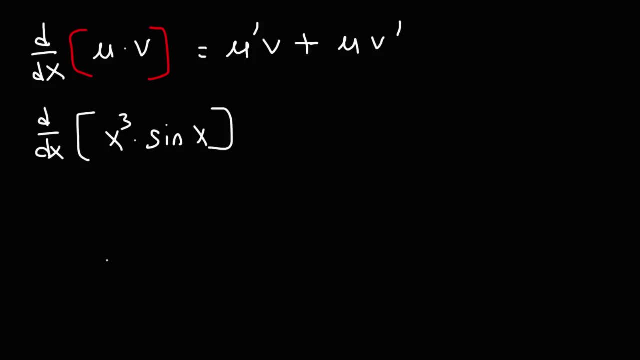 x cubed times sine x. In this example you could say that u is x cubed And v is sine x. So we're going to differentiate. the first part, That is x cubed. The derivative of x cubed is 3x squared. 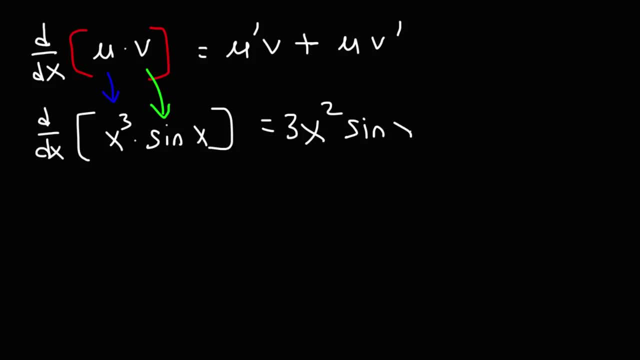 And then we're going to leave the second part the same. So we're just going to rewrite sine x Plus. now we're going to rewrite the first part- x cubed- And then take the derivative of the second part. 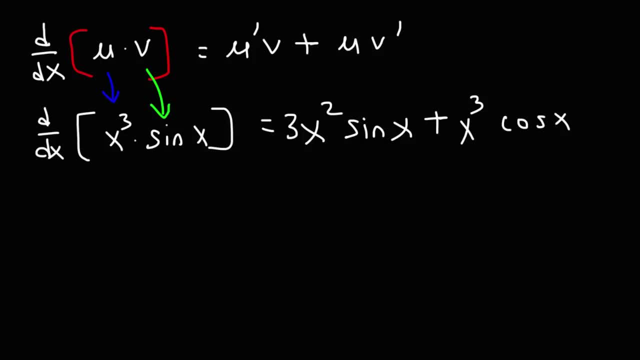 The derivative of sine x Is cosine x. So this is the answer. Now, for those of you who want to simplify it, you could factor out the GCF, Which is x squared. If you decide to do that, here's what you're going to get. 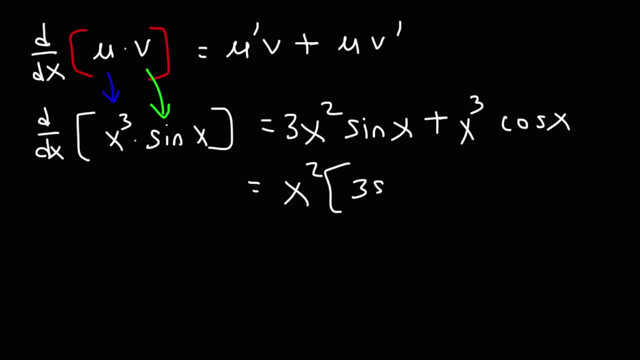 Taking out x squared in the first term, you'll be left with 3 sine x. Taking out x squared in the second term, you'll be left with x cosine x. So you could leave your answer in this format if you want to. 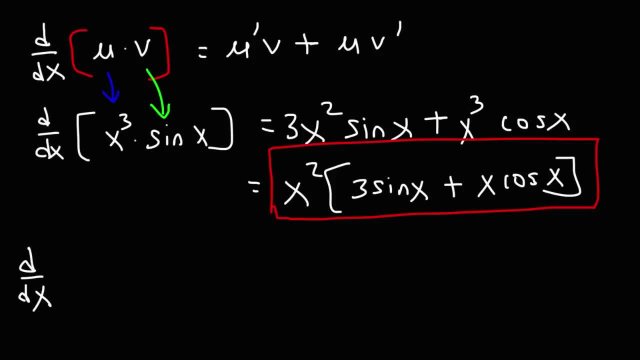 Now let's try another example. What is the derivative of x squared, ln, x. So feel free to pause the video if you want to try that. So this is u and this is v. So let's begin by differentiating the first part: x squared. 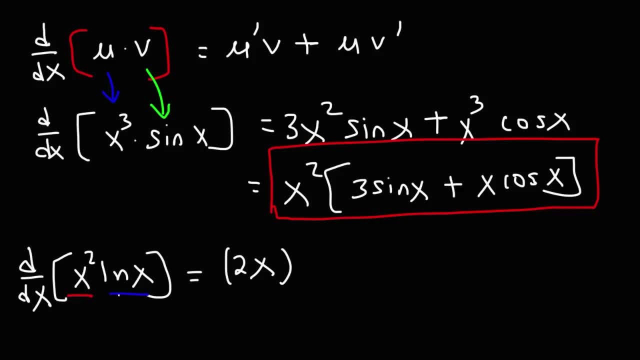 So we're going to get 2x And then we're going to rewrite the second part, ln, x. We're not going to change that. Plus, let's rewrite the first part- x squared- And then let's take the derivative of the second part. 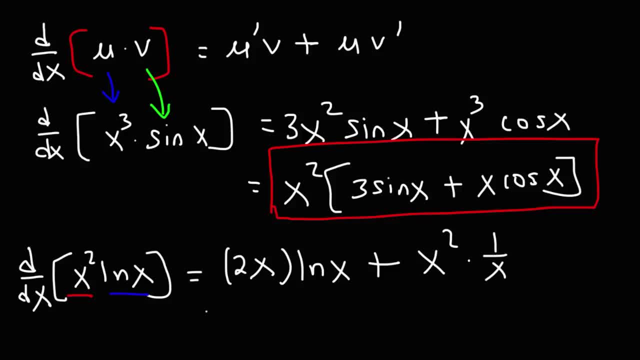 The derivative of ln x is 1 over x, So we're going to get 2x ln x And then x squared times 1 over x. that's like x squared divided by x, which is x. Now, like before, we can factor on x. 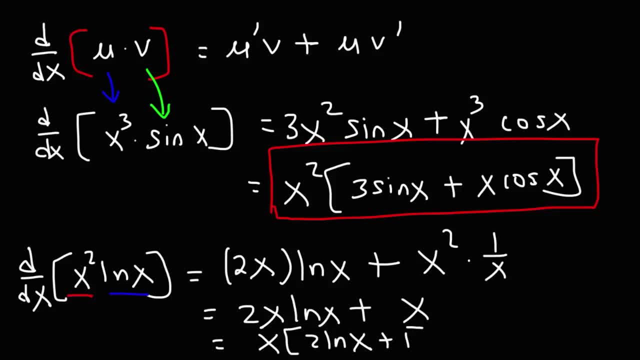 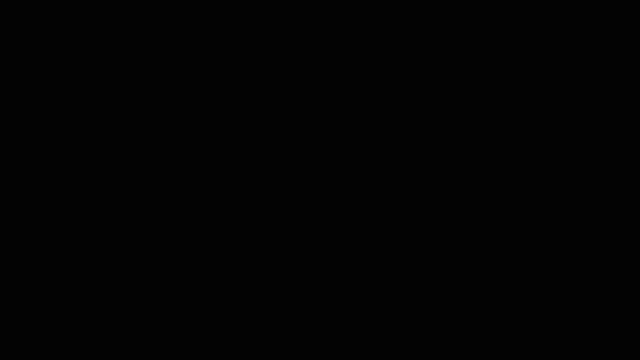 If we do so, we're going to get 2 ln x plus 1.. So that's the final answer, if we wish to simplify it that far. So now you know how to use the product rule when finding derivatives. Here's another example. 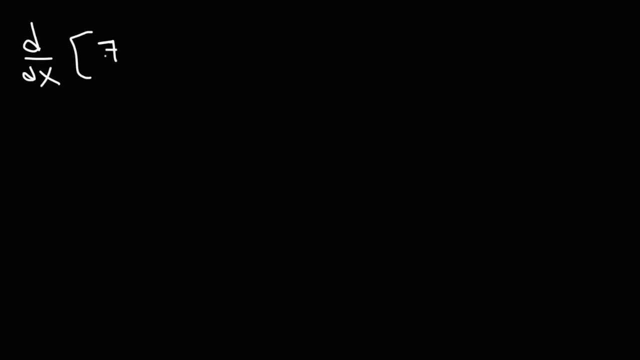 So let's say we have 7x plus 4 times x, squared plus 8. Now we could use the product rule to find the derivative of this expression. Or we can find the derivative of this expression, Or we can FOIL and then use the power rule to find the derivative of the resultant polynomial function. 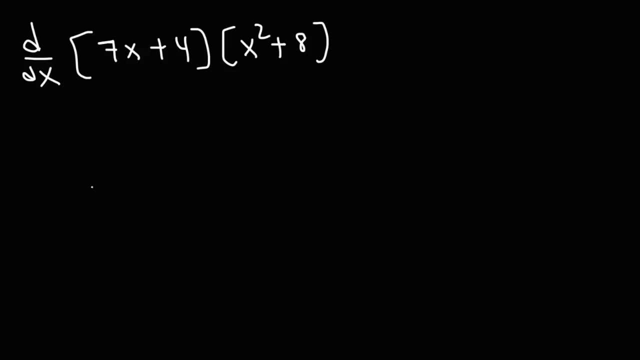 But let's use the product rule. So first let's find the derivative of the first part, 7x plus 4.. The derivative of 7x is 7.. The derivative of 4 is 0. So we just get 7.. 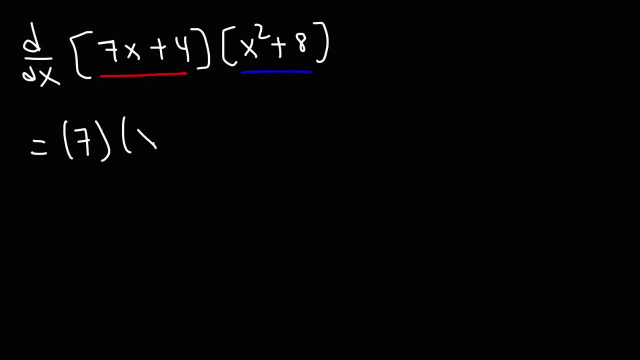 Next we're going to rewrite the second part And then we're going to rewrite the first part And then take the derivative of the second part. The derivative of x squared is 2x. The derivative of the constant 8 is 0.. 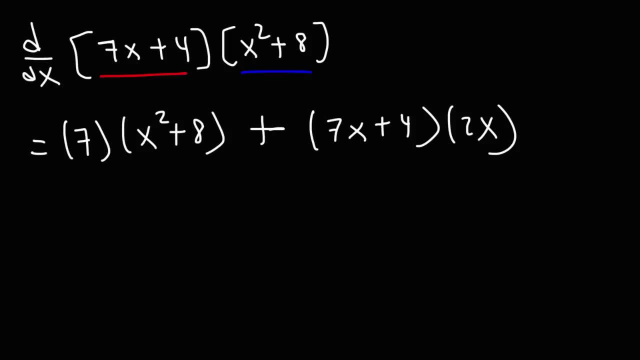 So this is the answer that we get. Now what I'm going to do is I'm going to distribute and combine like terms. So this is going to be 7x squared plus 56. And this is going to be 14x squared plus 8x. 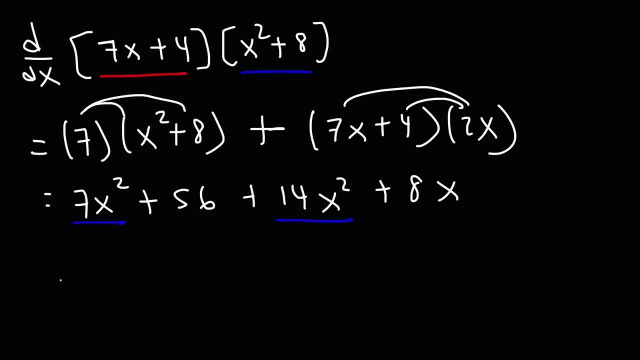 So I can combine like this: So I'm going to combine 7x squared and 14x squared, So I'm going to get 21x squared plus 8x plus 56.. And so this is the final answer. 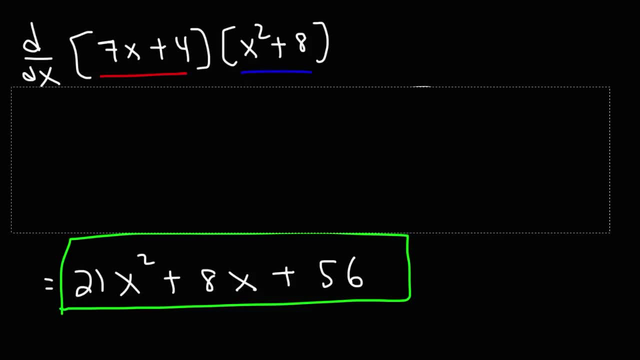 Now note the other way in which we can get the answer. We could have initially distributed, before we take the derivative: 7x times x squared is 7x cubed, And then this is 7x times 8, which is 56x. 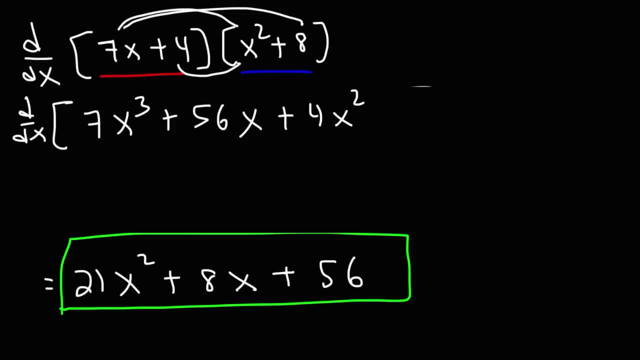 This is 4x squared, And this 4 times 8 is 32.. Now if we were to take the derivative of 7x cubed, that's going to be 7 times 3x squared, which is 21x squared. 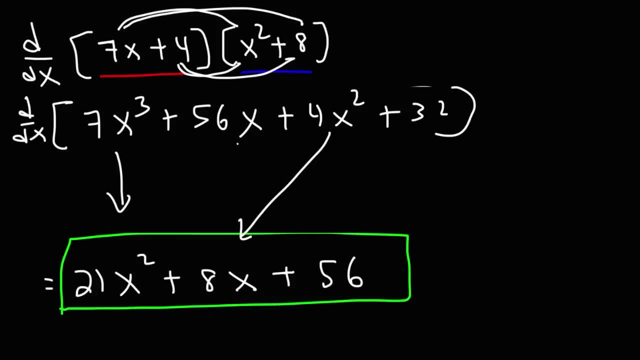 The derivative of 4x squared is 8x And the derivative of 56x is 56.. The derivative of the constant is 2x, So we would still get the same answer in the end. Now let's talk about the quotient rule. 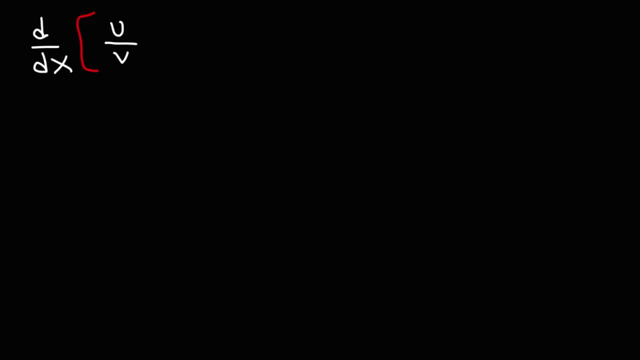 Let's say if we have a function divided by another function or u over v, To find the derivative of that expression we could use this formula: It's going to be v? u prime minus u, v prime over v squared. So let's say we want to find: 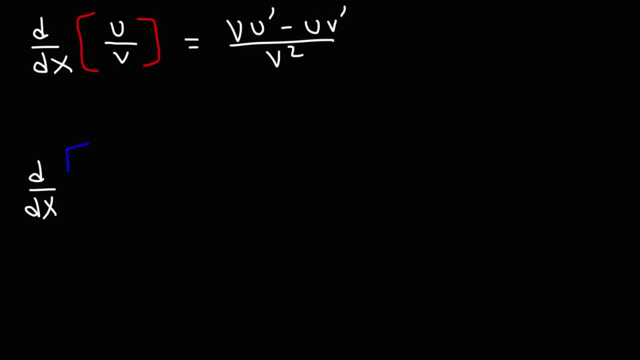 The derivative of 3x minus 5 over 7x plus 4.. Now, if you want to, it helps to write down a few things. So u is whatever is on the numerator of the fraction. So we could say that u is 3x minus 5.. 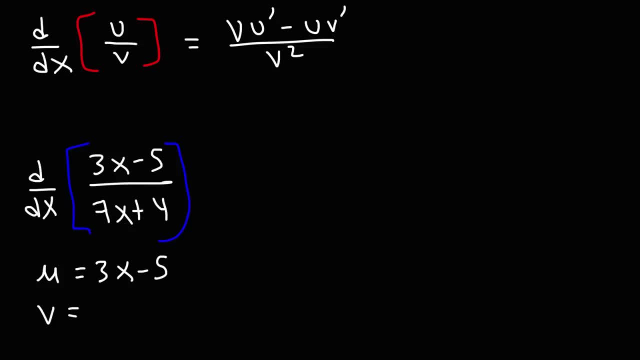 v is the stuff on the bottom or on the denominator of the fraction. So that's 7x plus 4. u prime, the derivative of 3x minus 5, is just 3. v prime in this example is simply 7.. 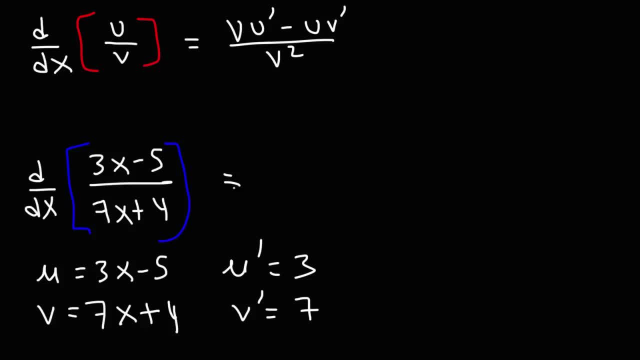 So now we just got to plug in everything into that formula. So it's v, that's 7x plus 4, times u prime, which is 3.. And then minus u, that's 3x minus 5, times v prime, which is 7.. 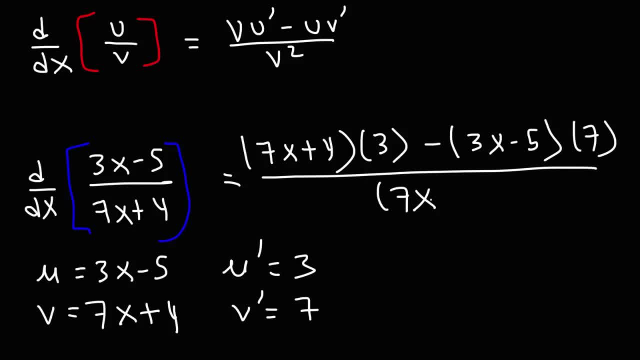 Divided by v squared, So that's 7x plus 4 squared. Now let's do some algebra. So let's begin by distributing the 3 to 7x and 4.. 7x times 3 is 21x. 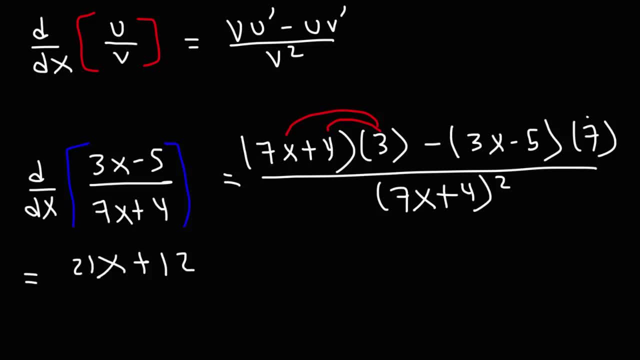 4 times 3 is 12.. Next let's distribute 7 to 3x and keep in mind it's a negative sign. So that's going to be negative 21x. And then 7 times, 7 times negative 5, combined with that negative sign, that's going to be positive 35.. 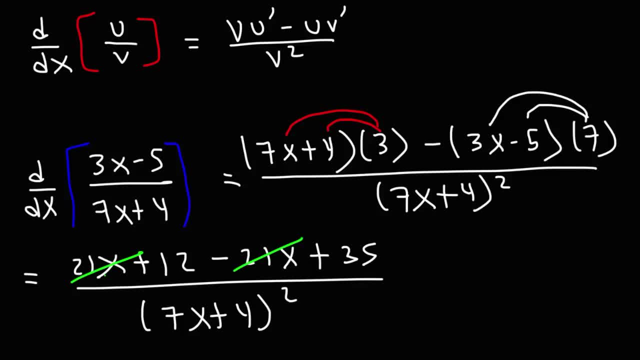 So immediately we could see that we could cancel the 21x And then we can combine 12 and 35, which will be 47. So the final answer is 47 divided by 7x plus 4 squared. for this problem, 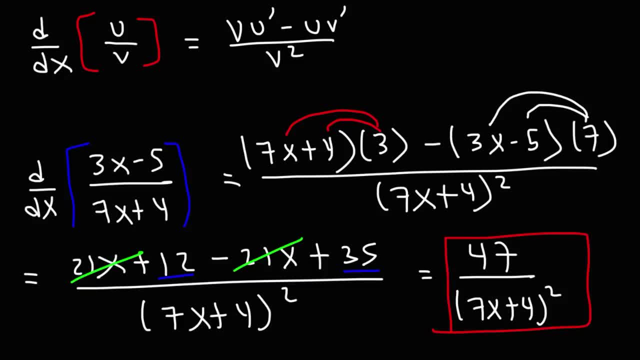 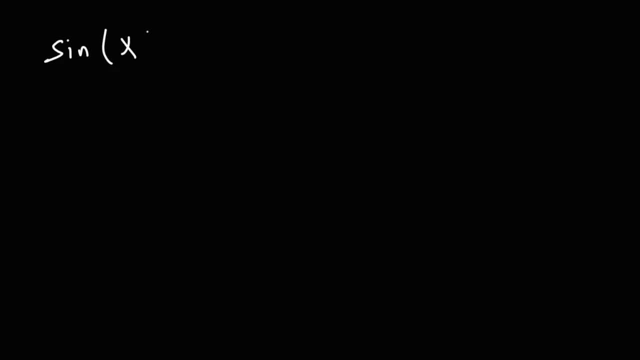 So that's how you can use the quotient rule Whenever you have a division of two functions. Now let's talk about the chain rule. We've covered some examples of it early in this video. What is the derivative of sine x to the 5th power? 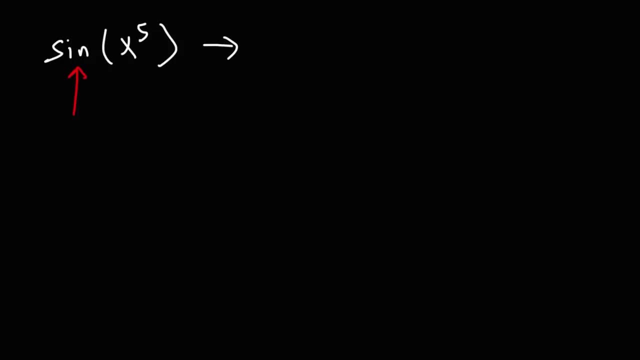 From what we talked about. we would differentiate the outer part of the function. The derivative of sine is cosine, And then we would keep the inside the same, And then we would differentiate the inside part of the function, The derivative of x to the 5th power. 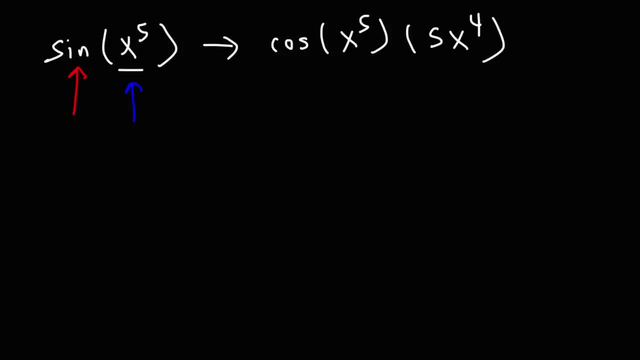 is 5x to the 4th power. That process can help you to solve derivatives associated with the chain rule. So when dealing with the chain rule, you're dealing with composite functions. So if you want to find the derivative, 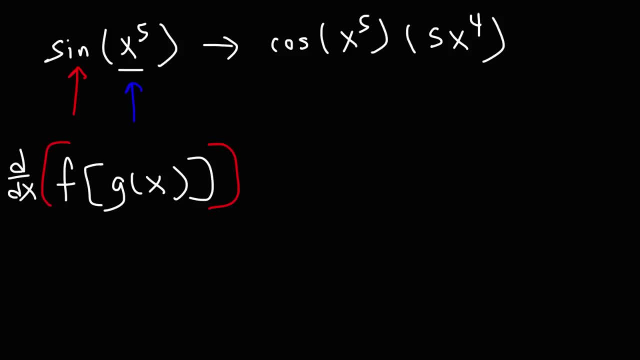 of a function inside of another function, like f of g of x, It's equal to the derivative of the outside function, So f prime, And then the inside function stays the same, That is g of x And then times the derivative. 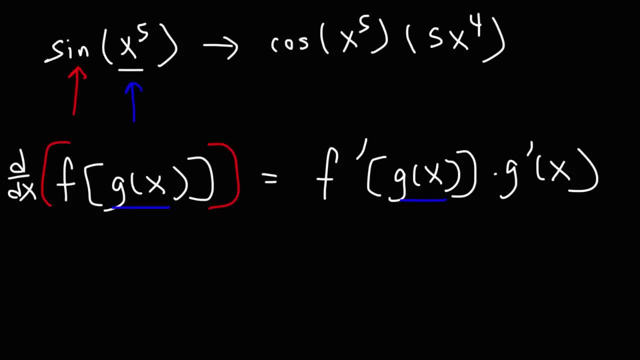 of the inside function, g, prime of x. So that's how you can find the derivative of a composite function When you have a function inside of another function. So let's say we want to find the derivative of 4x cubed. 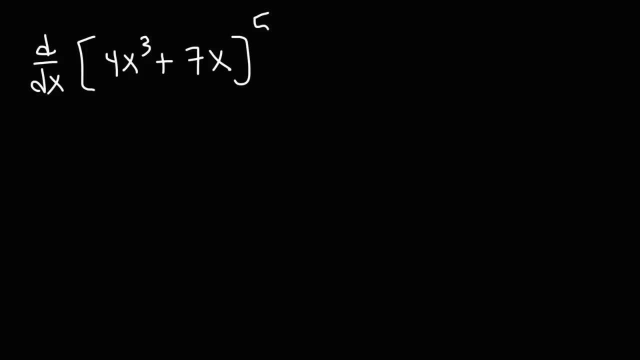 plus 7x, raised to the 5th power. In this case we need to start with the out of function. That is the power rule. So we're going to move the 5 to the front. We're going to keep the inside function the same. 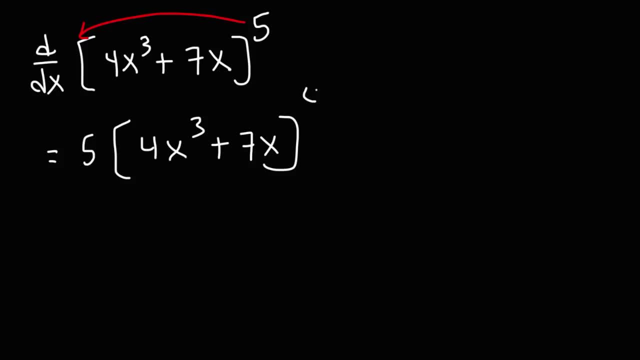 And then we're going to subtract the exponent by 1.. Next we're going to take the derivative of the inside function. The derivative of 4x cubed is 12x squared. The derivative of 7x. 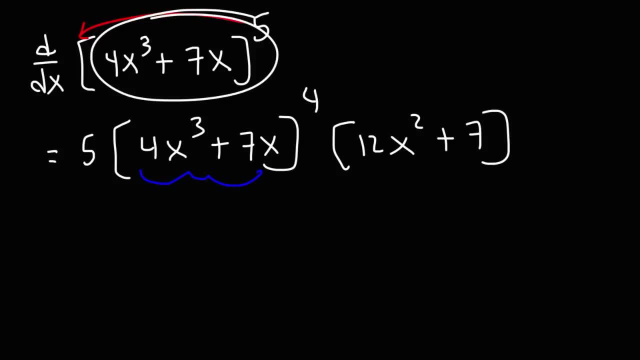 is 7.. So that's the derivative of this function. So you don't have to follow this 5 times. You can simply use the chain rule to get the answer. Now let's move on to our next example. 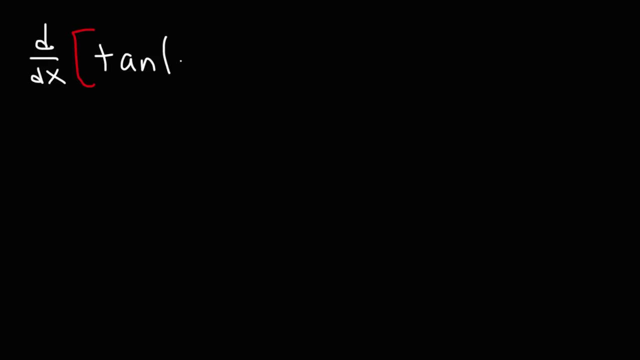 What is the derivative of tangent of sine x cubed? Go ahead and work on that example. So first we're going to find the derivative of the out of function tangent, And that's going to be secant squared. 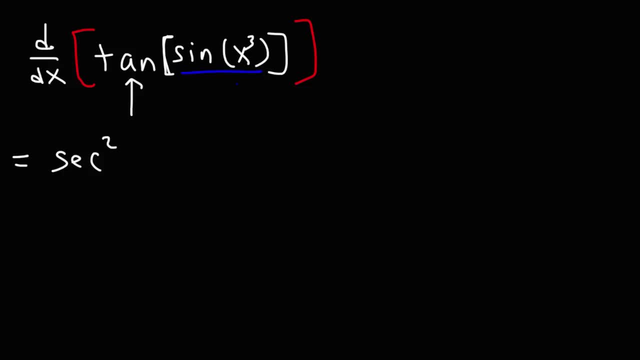 Now inside of tangent we have sine x cubed, So we're going to have the same thing inside of secant squared. So we're starting with the out of function and we're working our way in. 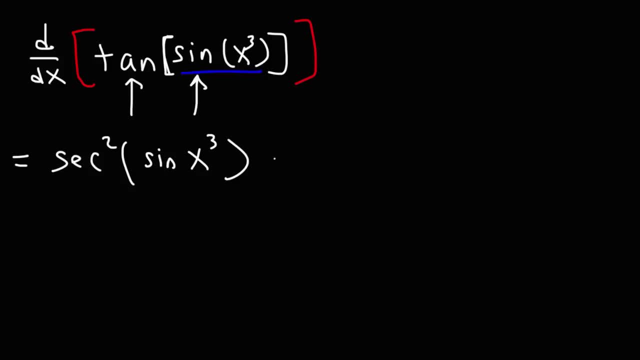 So now let's work our way in towards sine. The derivative of sine is cosine And the angle of sine is x cubed. So the angle of cosine will be x cubed. And then we're going to work even further. 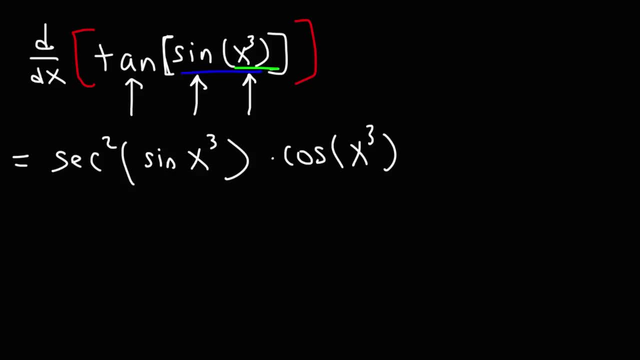 towards the inside part of the functions. The derivative of x cubed is 3x squared. Now, that's as far as we can go. So this is the answer of this expression: Secant squared sine x cubed. 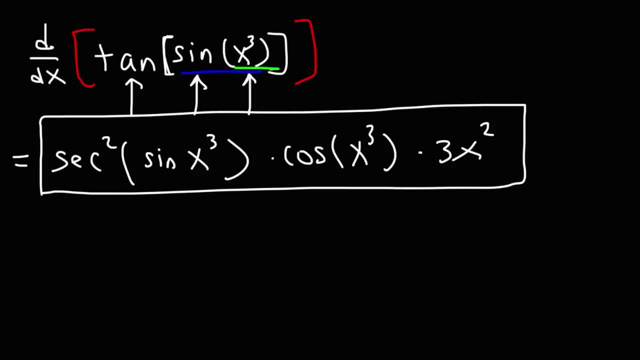 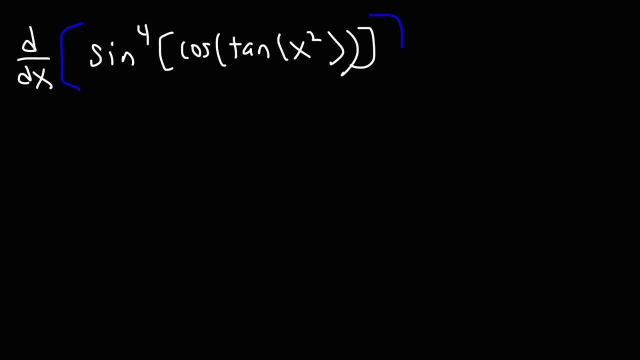 times cosine x cubed, times 3x squared. Here's another example we can work on: Find the derivative of sine to the fourth power of cosine of tangent x squared. Now what I would recommend doing, since we have an exponent here. 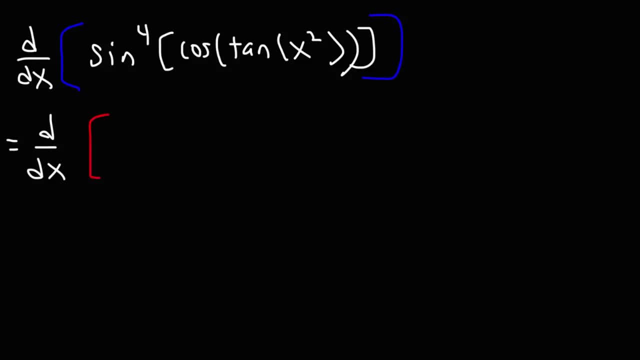 is rewriting the expression. So basically what this means is that this whole thing is raised to the fourth power And it affects the way you're going to apply the chain rule, Because before you can differentiate the sine function. 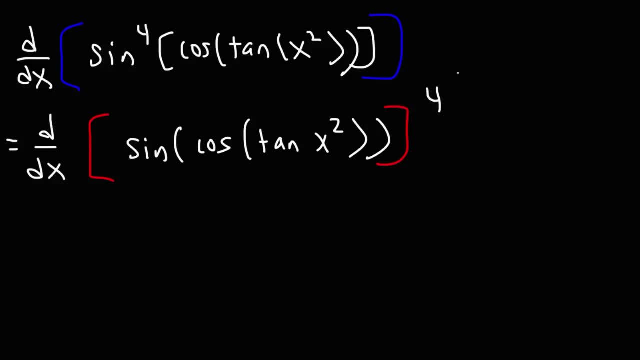 you need to use the power rule on that exponent. So let's move the 4 to the front, So it's going to be 4.. And then we're going to rewrite everything we see inside of the brackets highlighted. 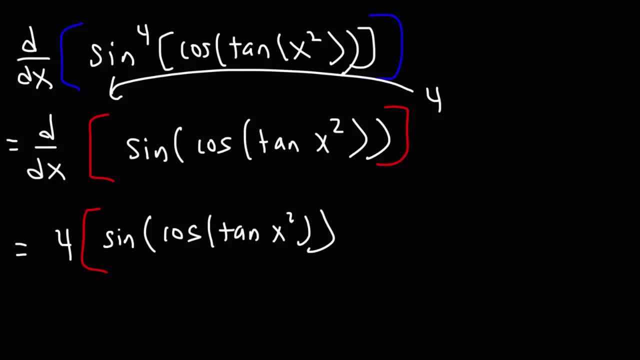 in red. Now we're going to subtract the exponent by 1. And then we're going to differentiate the sine function, So that's going to be cosine, And then the angle of sine is everything we see here. 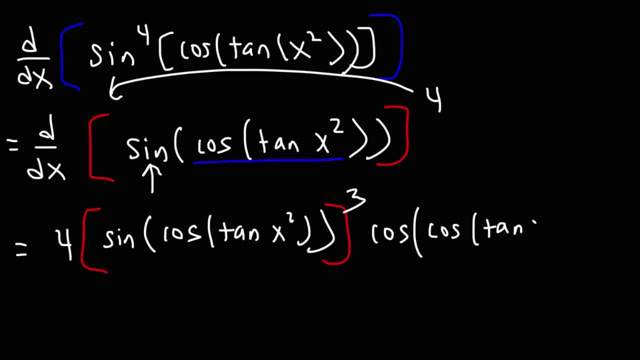 That's cosine of tangent x squared. So now we're going to move inward towards cosine. By the way, there's a multiplication for all of these functions, So it's times The derivative of cosine is negative sine. 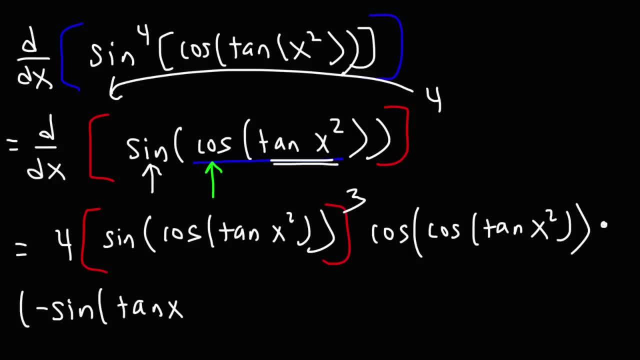 And the angle of cosine is tangent x squared. So we're going to rewrite that. Now let's work our way in towards tangent. The derivative of tangent is secant squared And the angle is x squared. Finally, we can. 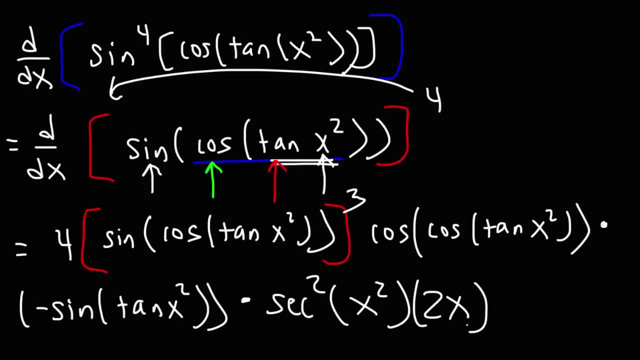 find the derivative of x squared, which is 2x, And so this whole thing is our final answer. Now, of course, you can combine a few things. You can combine the 4. and the 2x and the negative sine. 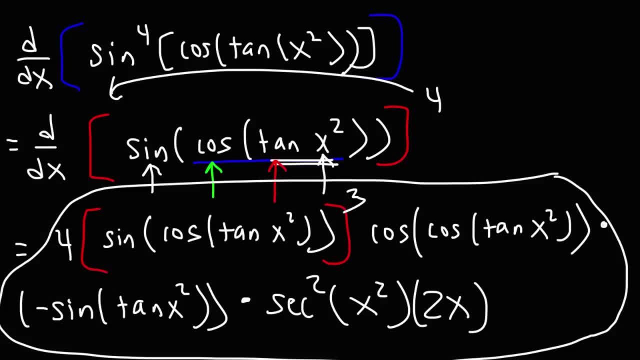 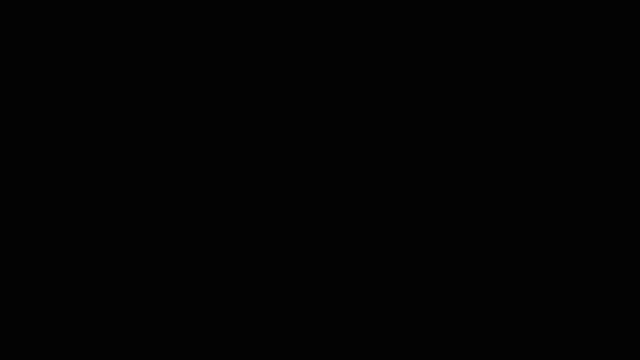 And you can put negative 8x in front. But besides that, there's nothing else you can do here. So that's it for this problem. Now, the next topic we need to talk about is implicit differentiation. Sometimes, 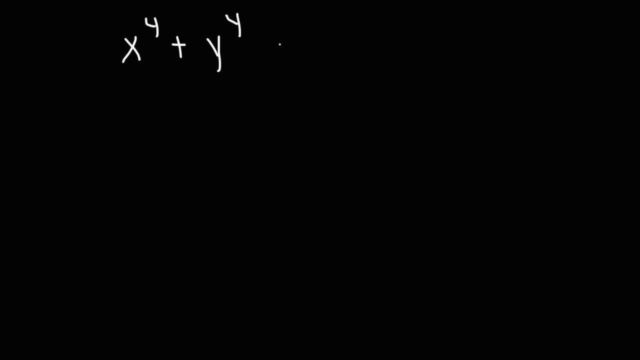 you'll have equations with two different variables Like this one: x and y, And you want to find the derivative of y with respect to x. So basically, you want to determine the value of dy dx. How do you do that? 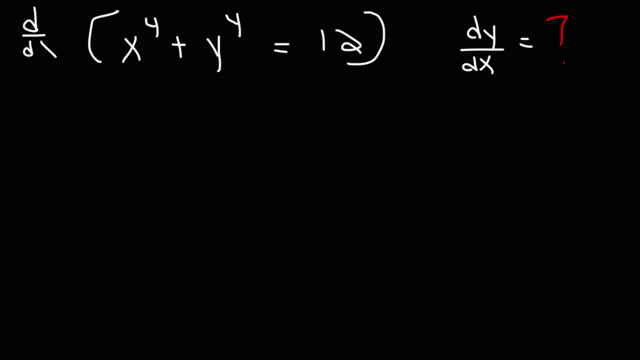 Well, what you do is you're going to differentiate both sides with respect to x. Now, before we do that, I want to talk about a few things. When you differentiate x cubed with respect to x, you're going to get 3x squared. 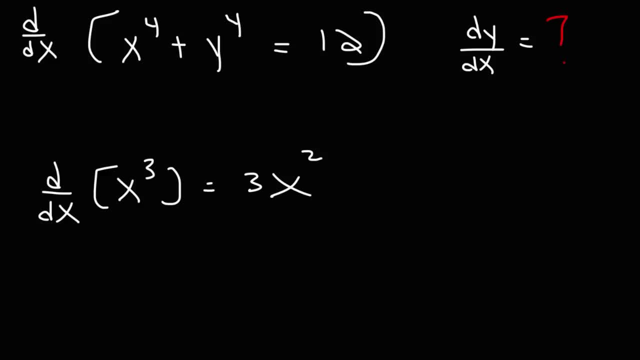 And technically you get times dx over dx, which cancels to 1.. But if you want to differentiate y cubed with respect to x, you're going to get 3y squared but times dy dx. 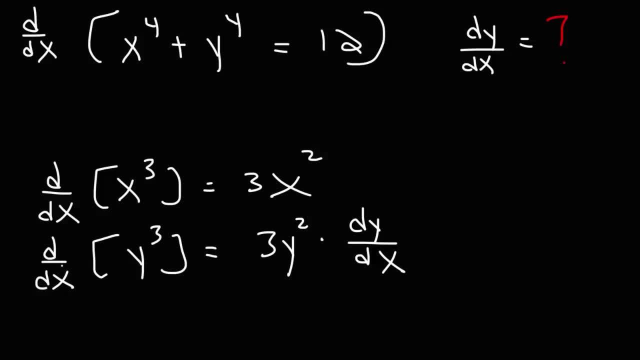 Note the difference here, Since these variables don't match up Here, these they do match up. So this would be dx over dx, which is pointless in writing, So implicit. when dealing with implicit differentiation problems, every time you differentiate y. 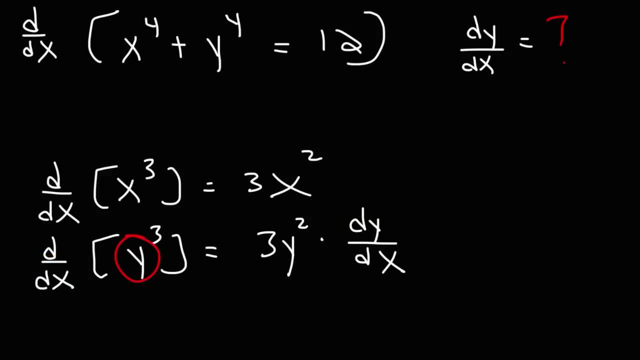 with respect to x. you need to add dy, dx. Now sometimes you'll be dealing with what is known as related rates. Instead of differentiating with respect to x, you'll be differentiating with respect to t or time. 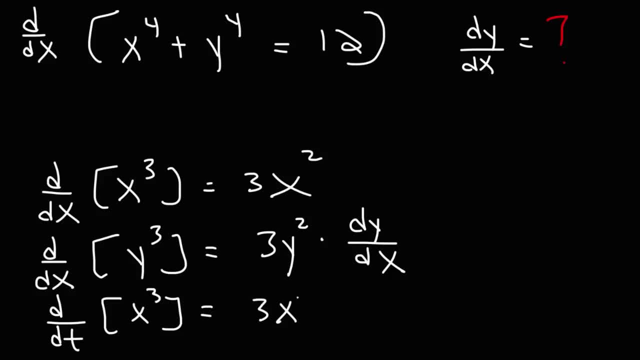 So if you differentiate x cubed with respect to time, it's going to be 3x squared, but times dx dt. Likewise, if you differentiate y cubed with respect to time, it's going to be 3y squared. 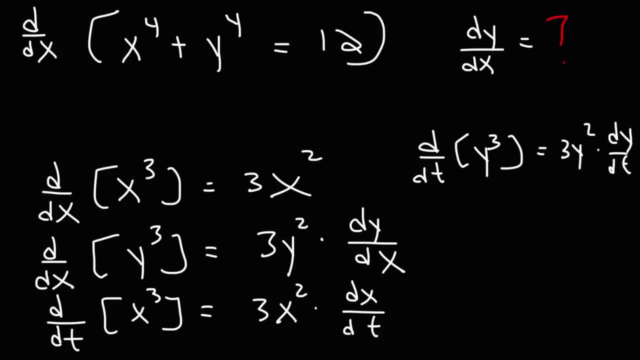 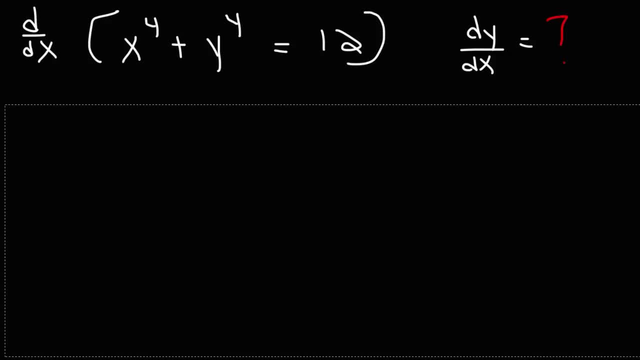 times dy, dt. So just keep that in mind. But when dealing with implicit differentiating, I mean, let me say that again, When dealing with implicit differentiation, we are differentiating with respect to x, So the derivative, 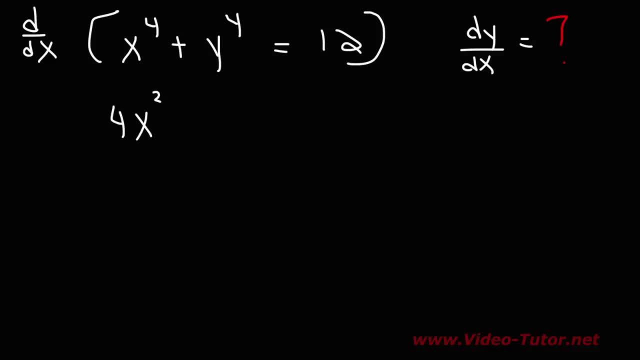 of x to the fourth is simply going to be 4x cubed, But the derivative of y to the fourth is going to be 4y cubed, but times dy over dx, And this is what we need to solve for. 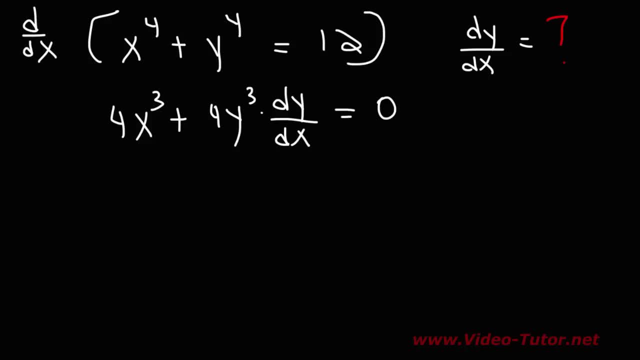 The derivative of 12 is 0. So I'm going to take this term and move it to the other side. So I'm going to have 4y cubed times dy dx, And that's can be equal to negative 4x cubed. 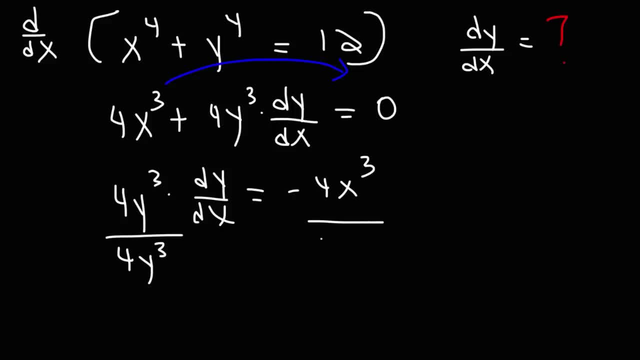 And then all we need to do is divide both sides by 4y cubed, And then the fours will cancel, And so we get dy over. dx is equal to negative x cubed over y cubed. 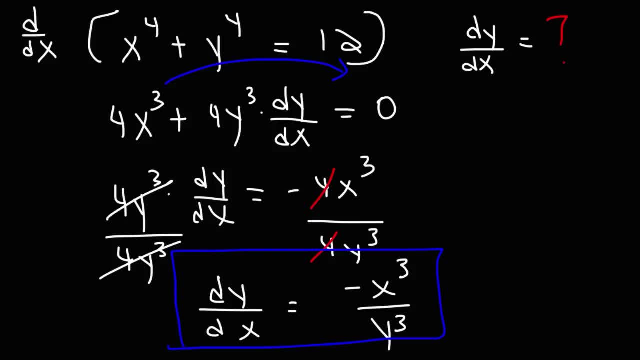 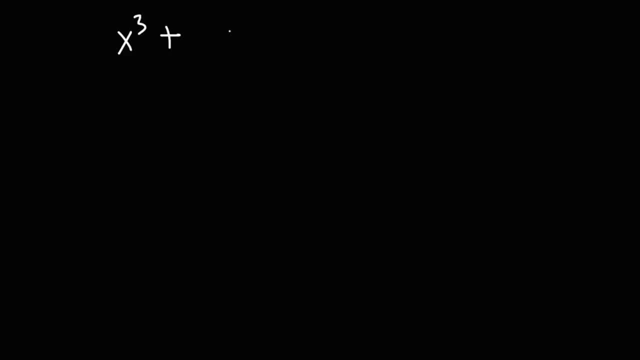 So that's a quick and simple example of how to perform implicit differentiation. For the sake of practice, let's work on one more example. Let's say we have x cubed plus 4xy plus y, squared is equal to 9.. 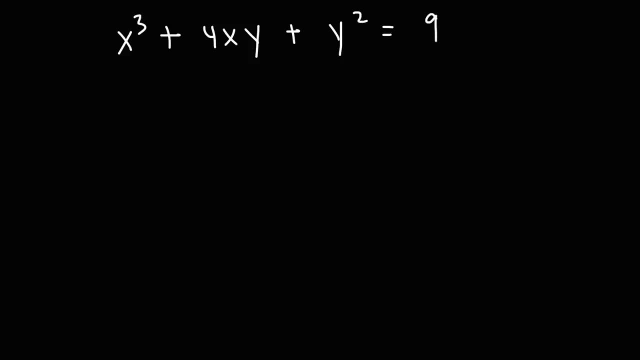 Go ahead and calculate the value of dy over dx. So we're going to differentiate this entire equation. with respect to x, The derivative of x cubed is 3x squared. Now notice that we have x and y. 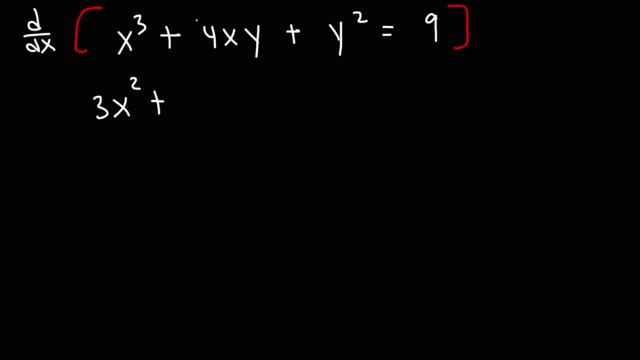 So we need to use the product rule. I'm going to say the first part, the u part, and the v part is going to be y. So the derivative of the first part, 4x, is just 4.. 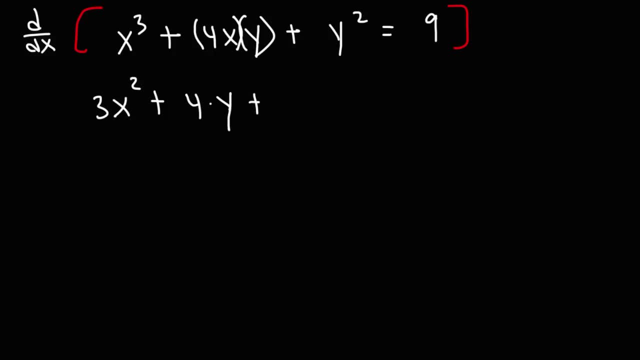 times the second part, which is just y plus the first part, 4x times the derivative of the second part. The derivative of y is going to be 1.. times dy over dx, Because we're differentiating y. 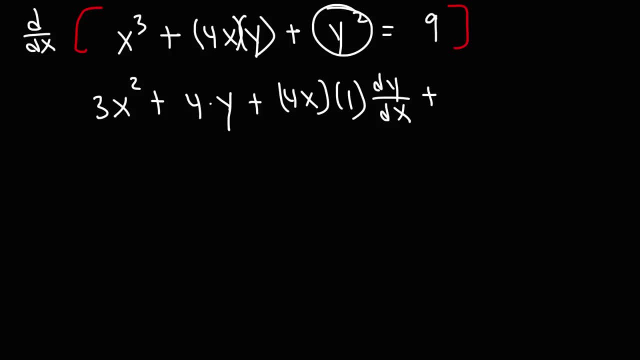 with respect to x. Now the derivative of y squared is going to be 2y times dy over dx, And the derivative of a constant is always 0.. So everything that does not have a dy over dx. 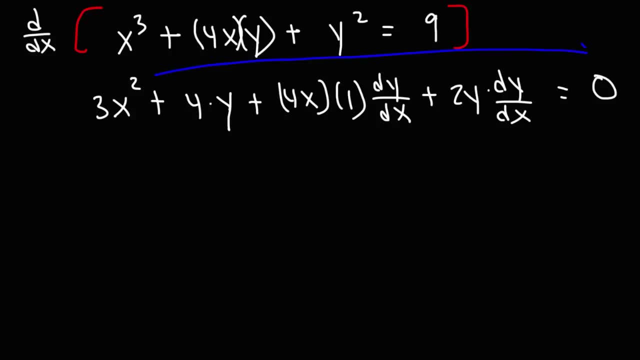 attached to it. I'm going to move to the other side. So I'm going to move these two terms across the equal sign. So we're going to have 4x dy over dx plus 2y. 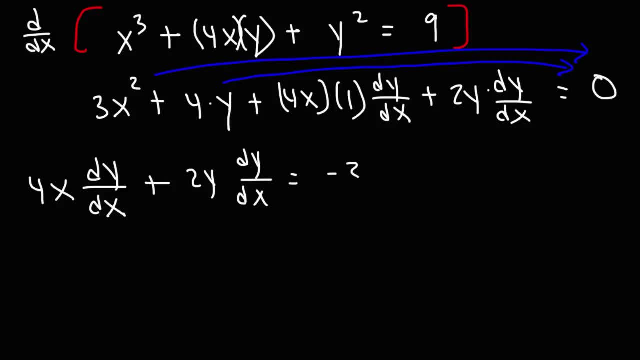 dy over dx And that's going to equal negative 3x squared minus 4y. So because we have a common factor, we can now factor out the dy over dx on the left side, And that's going to leave us with 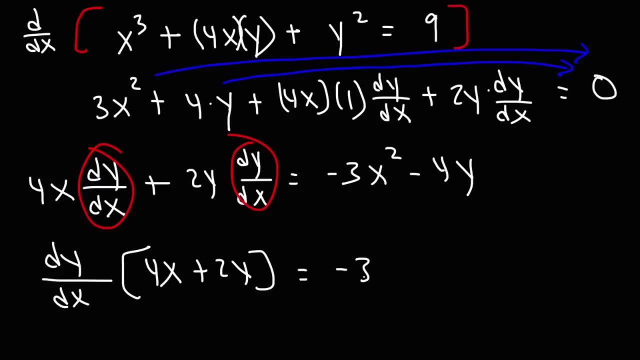 4x plus 2y, which equals negative 3x minus 4y. So now we can divide both sides by this 4x plus 2y. So these two will cancel And thus 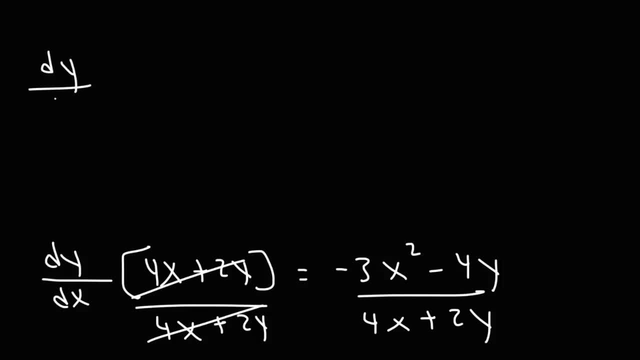 we have our final answer: dy over dx is equal to negative 3x squared minus 4y And we can factor out a 2 on the bottom. but I'm not going to worry about that in this example. 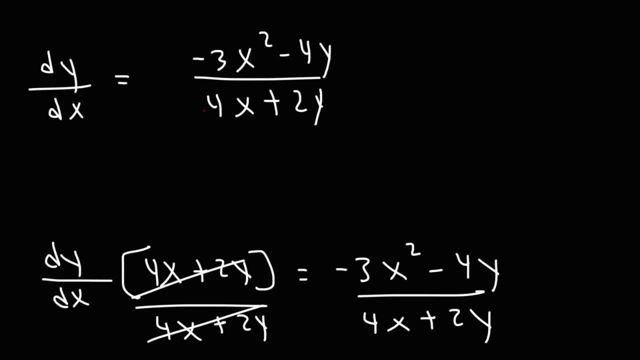 So that's going to be divided by 4x plus 2y. So now you know how to find the derivative in or using implicit differentiation. So far we talked about how we could find the derivative. 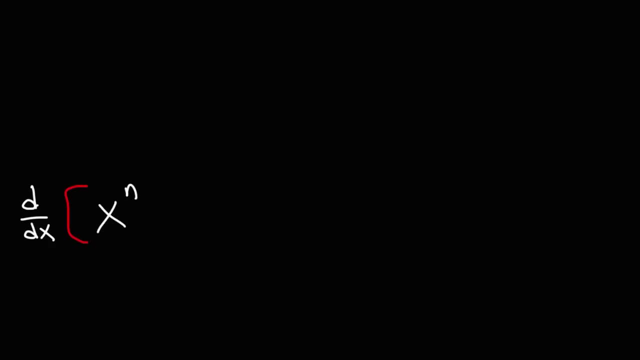 of a variable raised to a constant, And that is by using the power rule x to the n. the derivative of that is going to be n times x raised to the n minus 1.. And we also talk about having or finding the derivative. 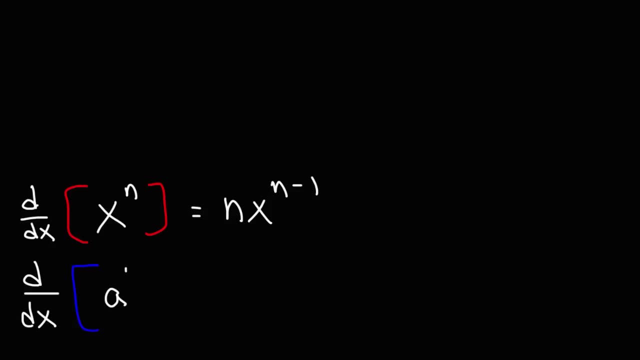 of a constant raised to a variable, And that was a to the u times u, prime times ln a. So we have a variable raised to a constant and a constant raised to a variable. But what about finding the derivative? 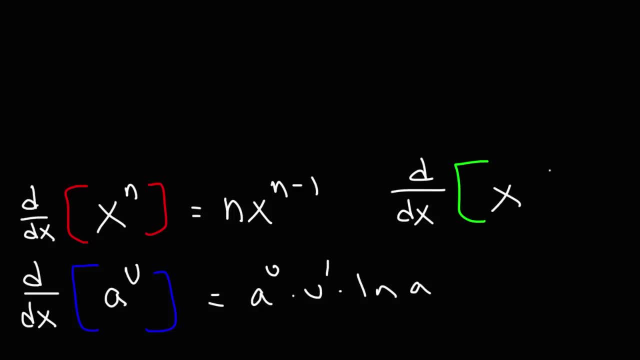 of a variable raised to a variable. How do we do that? How do we find the derivative of x raised to the x? Well, first let's make y equal to x raised to the x. So if we could find the derivative of y, 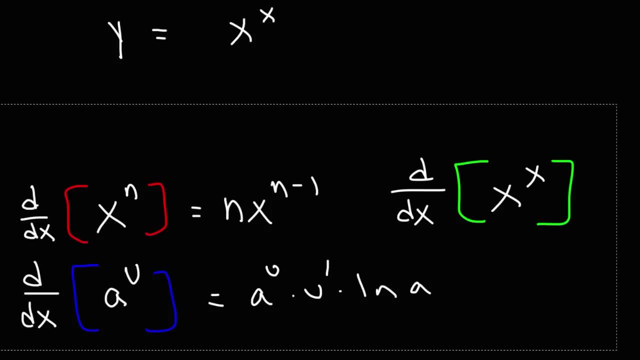 then we know what the derivative of x to the x is. That's step one. Step two is to take the natural log of both sides, So ln y is equal to ln x, raised to the x, Now a property of: 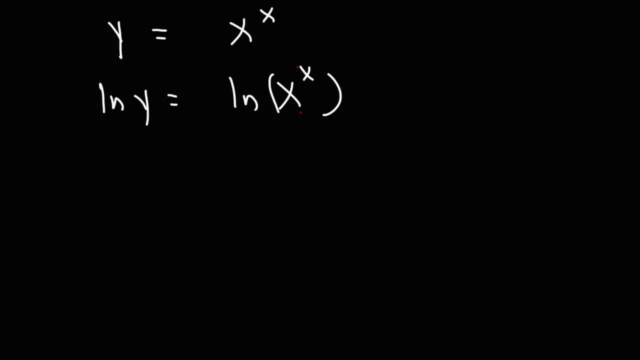 natural logs allows us to move the variable x to the front, And so what we're going to have is: ln y is equal to x, ln x, And now, at this point, we are going to differentiate both sides with respect to x. 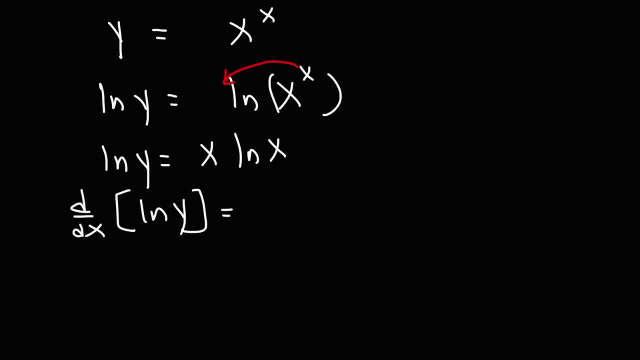 So here's how you can express that in mathematical words. Now we know that the derivative of ln x is 1 over x, So the derivative of ln y is going to be 1 over y. Now notice that we're differentiating y. 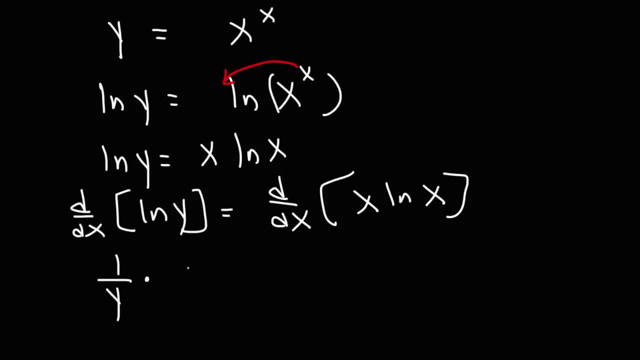 with respect to x. So when you see that you need to add dy over dx- This is basically implicit differentiation On the right side- we need to use the product rule. So we're going to differentiate the first part, x, which is 1.. 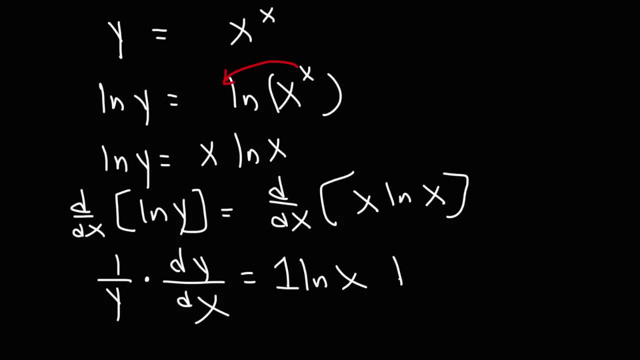 and leave the second part by itself, And then we're going to leave the first part by itself and then differentiate the second part. The derivative of ln x is 1 over x, So what we have now is 1 over y. 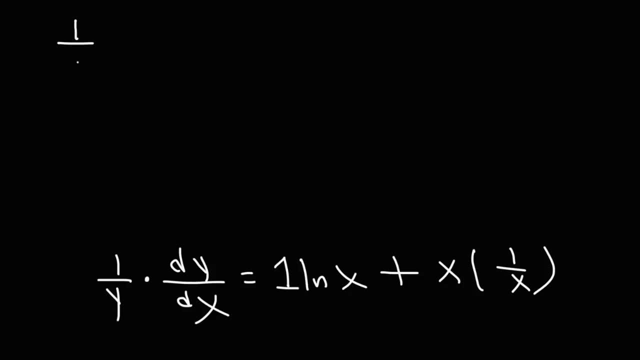 times dy over dx, And that's equal to ln, x, And then x times 1 over x. you can cross out the x variables, So it becomes plus 1.. And now what we're going to do is: 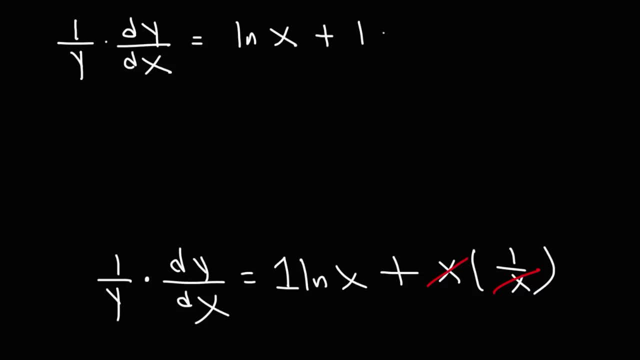 we're going to multiply both sides by y, So we can cross out the x variables, So it becomes plus 1.. And now what we're going to do is so we can cross out the y variables here. 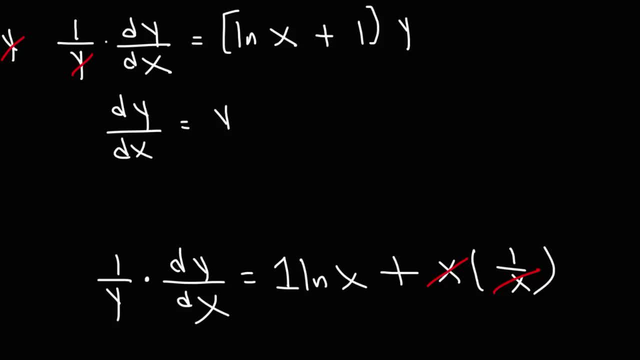 So we're going to have dy over. dx is equal to y times. you can say ln x plus 1.. or you can say 1 plus ln x. Now recall: at the beginning we said: x raised to the x is equal to y. 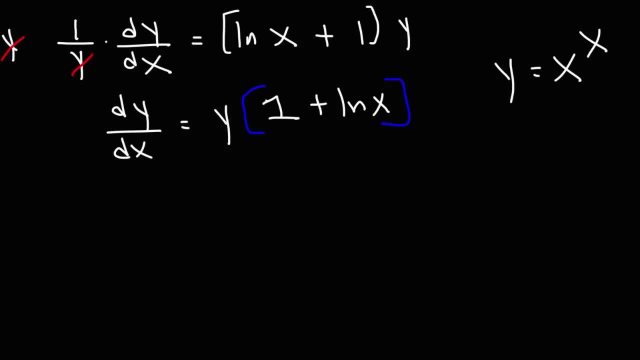 At this point we're going to substitute y with x raised to the x, So the final answer is going to be x raised to the x times 1 plus ln x. So that's how you could perform. 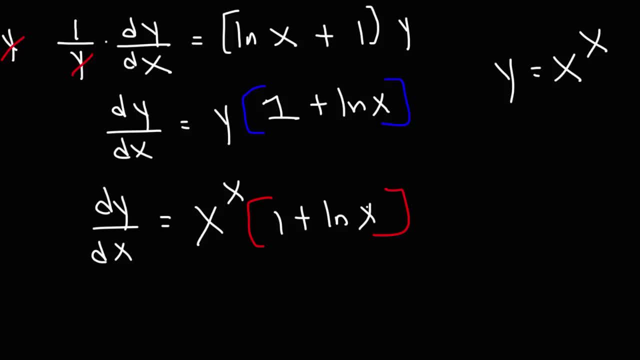 what is known as logarithmic differentiation. That's how you could find the derivative of a variable raised to a variable. So this is the answer. So you could say that the derivative of x raised to the x in this example,